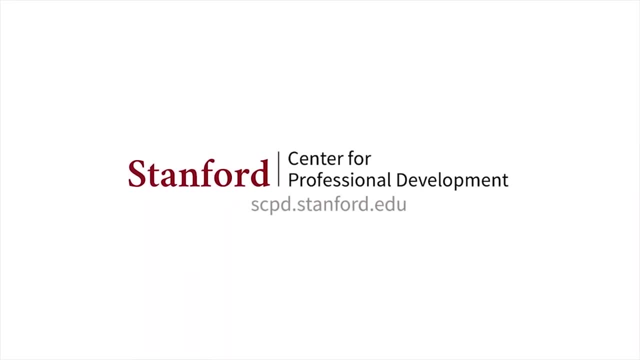 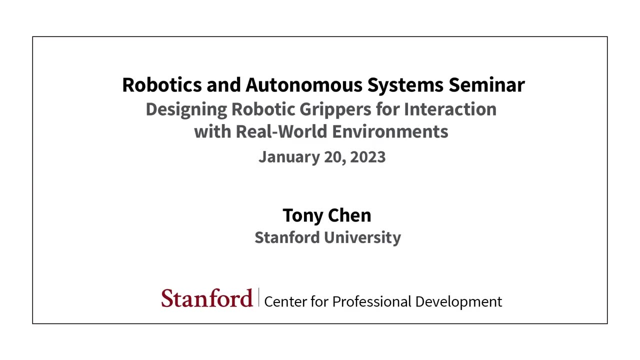 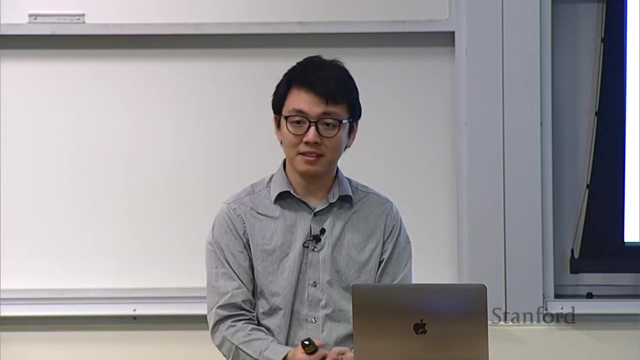 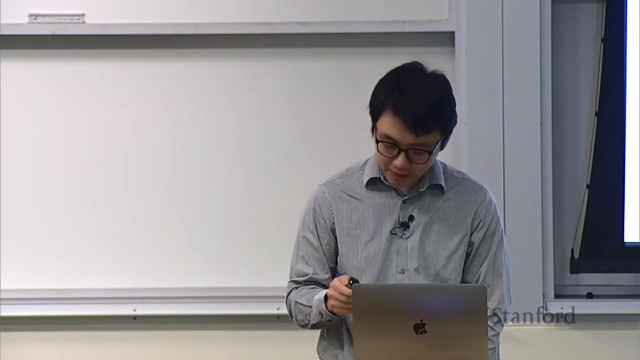 Thank you, Mark, for the introduction. My name is Tony Chen and I'm a six-year PhD student in Mark's lab, Biomimetics and Dextrose Mutilation Lab, and today I want to talk about designing robotic grippers for interaction with real-world environments. So a little bit teaser here. 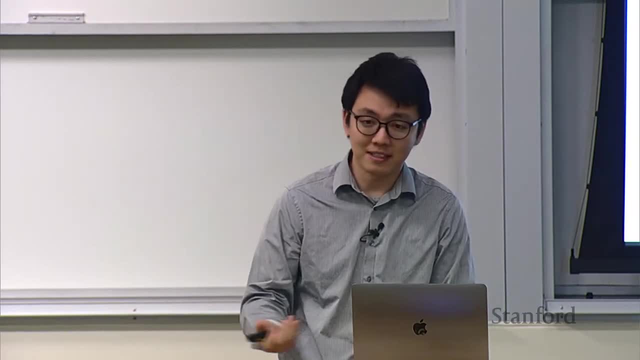 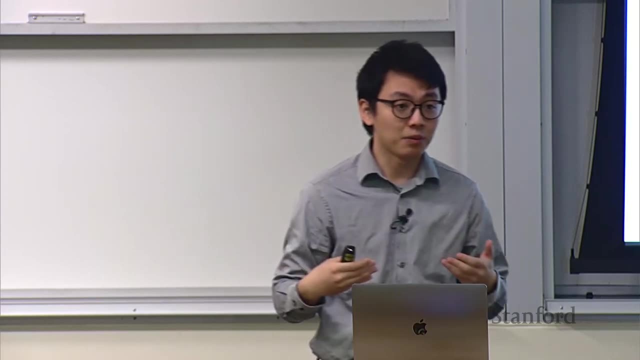 is robots, while we have robots around for 50,, 60,, 70 years now, all the way from the beginning in 1966 here at the Shakey, we always have platforms that can start with observation. We see what environment we want to deploy the robots in. In this case it's a hallway. 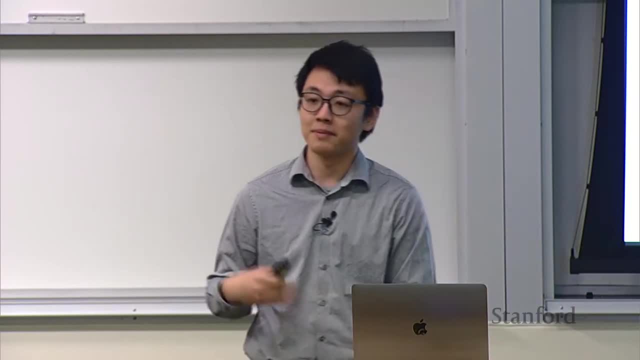 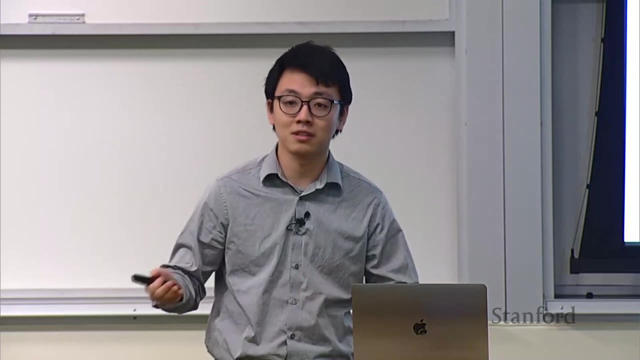 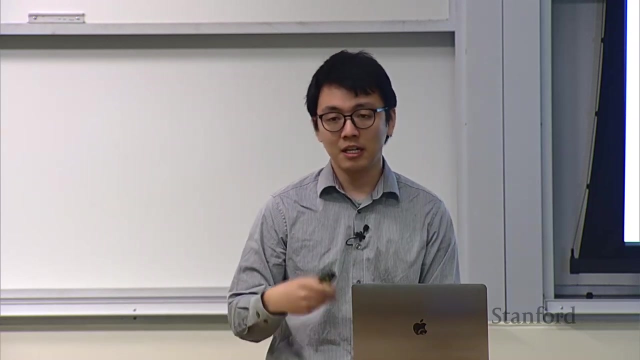 it's a cluttered room and we're equipping these robots with mobility, with a form of mobility. in this case, Let's have a bunch of sensors on there. see what obstacles in the way As the technology for certain robotic platforms mature more and more, then we start looking. 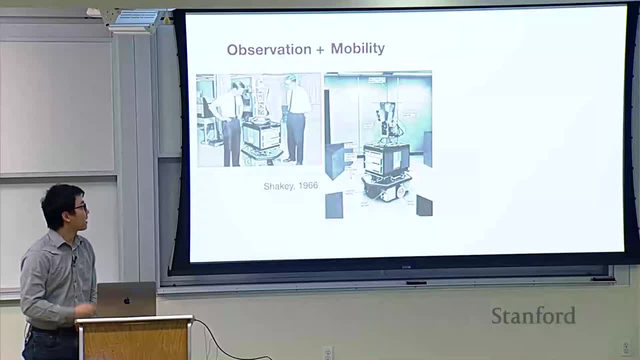 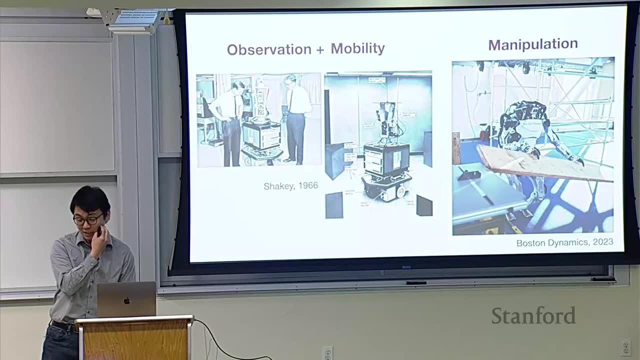 into how do we make these robots more useful. Then it comes to manipulation. So this is a screenshot of the new Boston Dynamics Atlas video that released a couple of days ago. Amazing, like a robot platform that can parkour and a lot of amazing mobility things. but 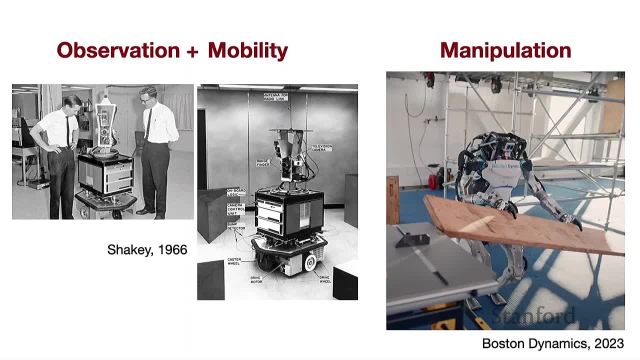 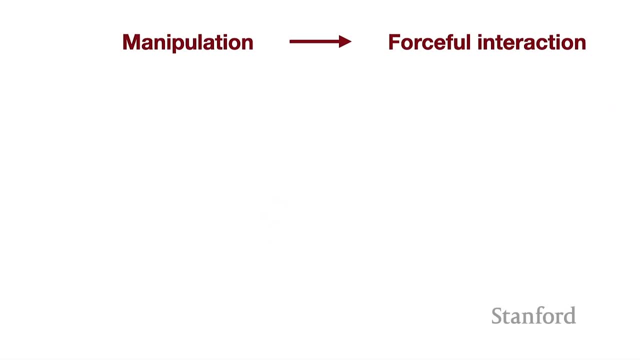 now, let's then. the next step is: let's try to put a gripper on there. Let's actually have it to manipulate. So what is manipulation? Manipulation is the way for the capability, to give capability to the robot to be able to forcefully interact with its environment, whether that be the 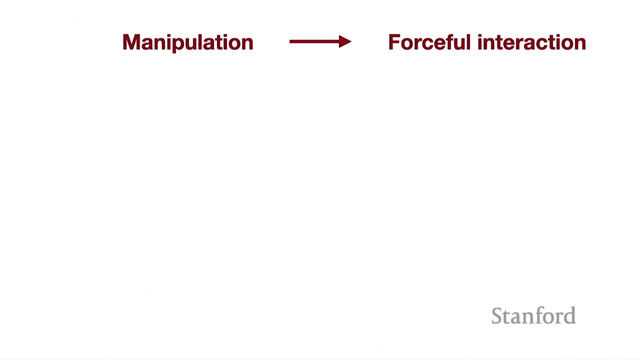 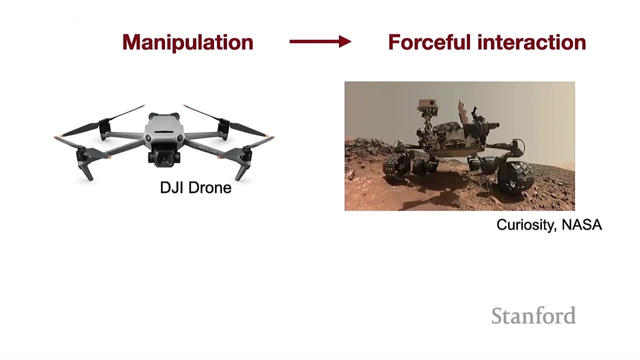 real-world environment or another object. So today, since I only have 20 minutes, I want to focus on two projects that worked on here on two other robotic platforms. One is a drone, the other one is a planetary exploration robot, And both of these robots are very similar. They're very similar in the way that they're. 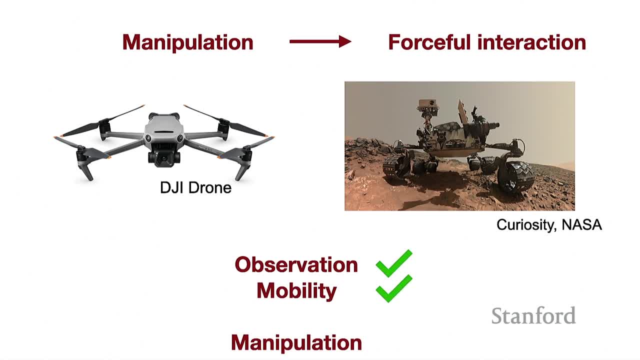 moving. They have these in both cases: observation and mobility. They do pretty well, especially for a drone. It's amazing parallel versatility in terms of observing and taking videos and stuff like that. But how do we add the capability to manipulate to these robotic platforms? 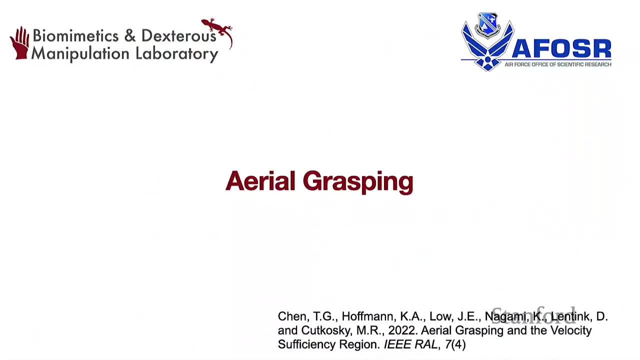 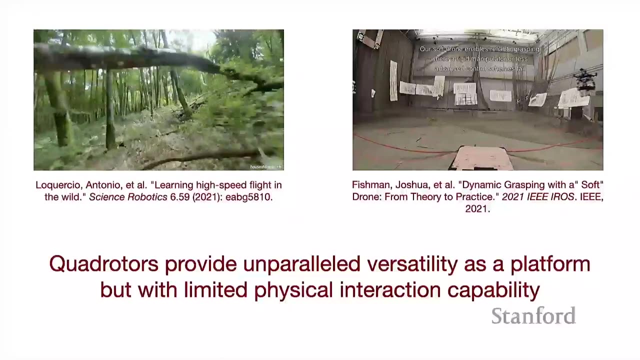 So first let's talk about drones, So aerial grasping. this work is done with me and collaborator Kenneth right here and it's funded by the Air Force And quite a lot of these drones really have a lot of good versatility as a robotic platform, But right now it's still 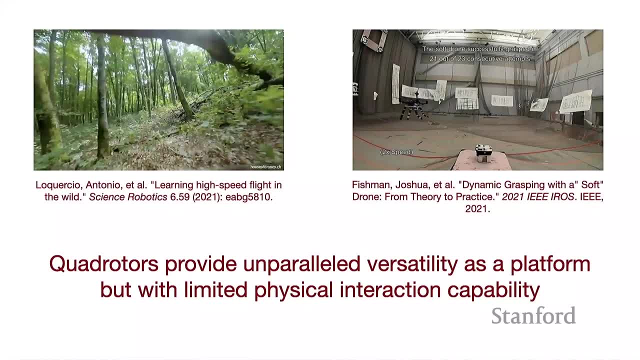 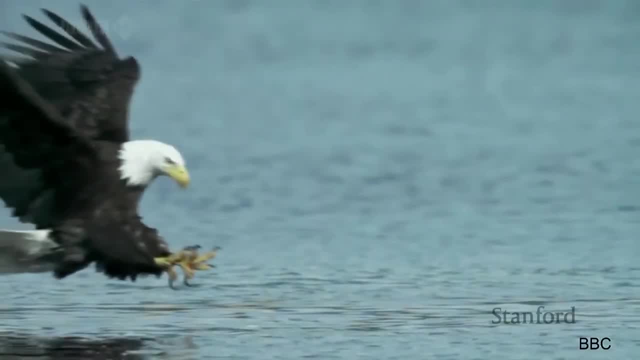 very limited in what interaction you can have with the real-world environment, So this is sort of state-of-the-art. what can drones do? But what can nature do? What has nature been doing for millions of years? at this point, Flying creatures like this eagle can catch. 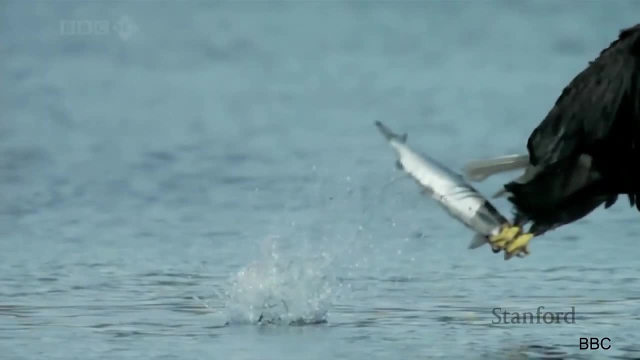 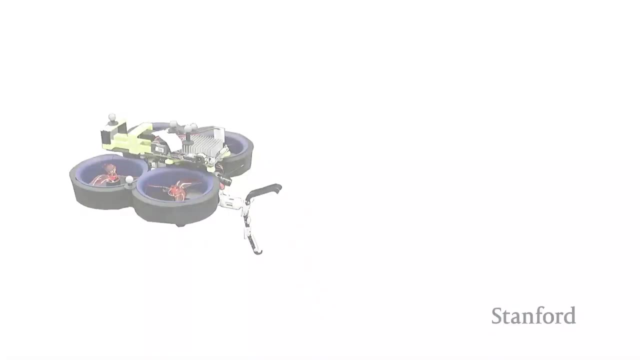 a fish out of the water like this. So when and how can we equip drones right now with technology that allows us to do something similar to this? Well, first of all, we need to be able to work towards it. The challenging thing about 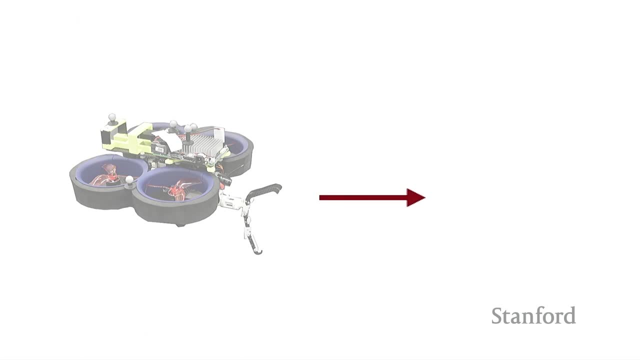 aerial grasping is that when you have a drone like this, you want to hit something mid-air, It's going to impart a large angular and linear disturbance to the system. Then how do you develop control strategies that can actually compensate for this and make sure the drone 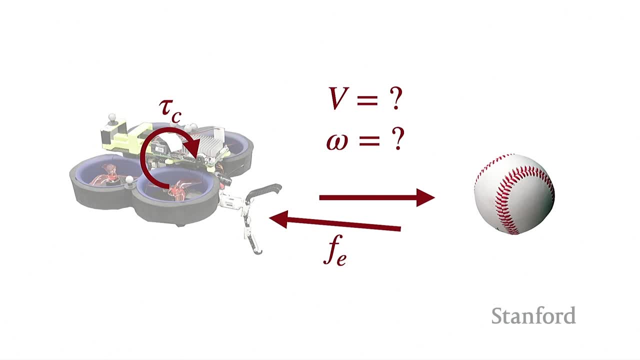 doesn't crash, make sure that it's at the right velocity or position profile to be able to capture the target. All this is to be seen. So where do we start Designing any gripper? To design any gripper, you need to have a. 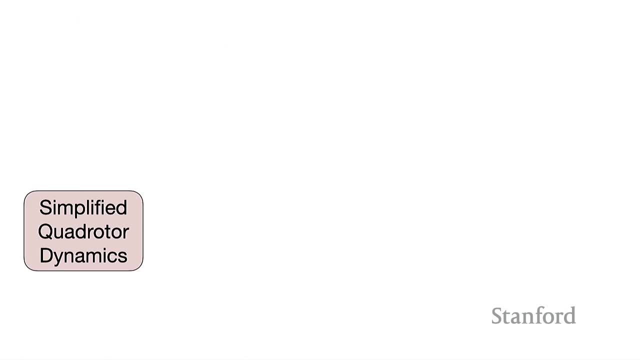 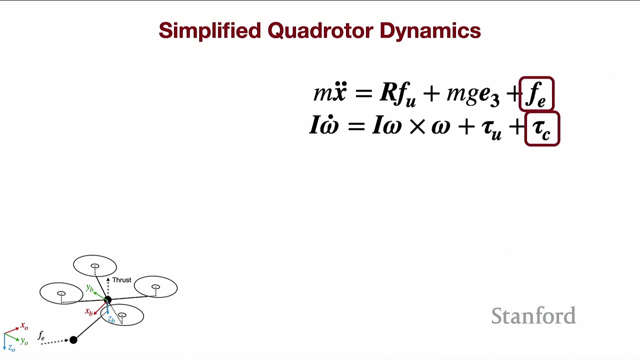 gripper to design anything to use in robots. We always start with dynamics. So here we actually employ a very, very simple quad-rotor dynamic model where the FE here and then TAL-C is the input force and torque due to the collision. These are related to each other through the 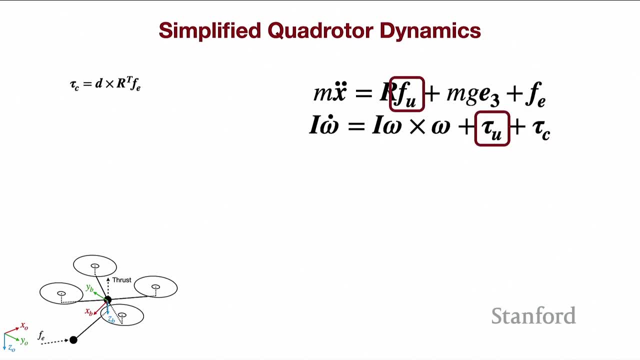 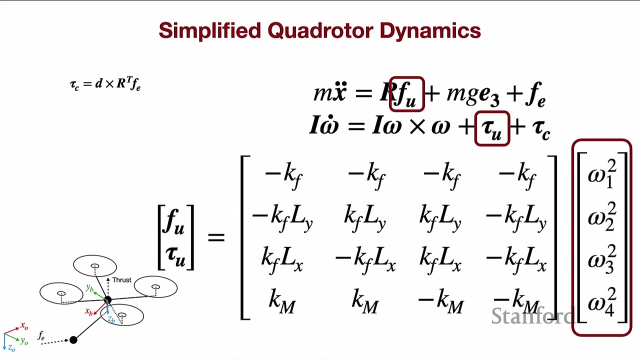 drone geometry, The F subscript U and TAL-U. here is basically the drone controller input- What force and torque is desired- And through a simple feedback policy and as a best-case approximation we can say: okay, they're related to the rotor speed. because all in all, that's. 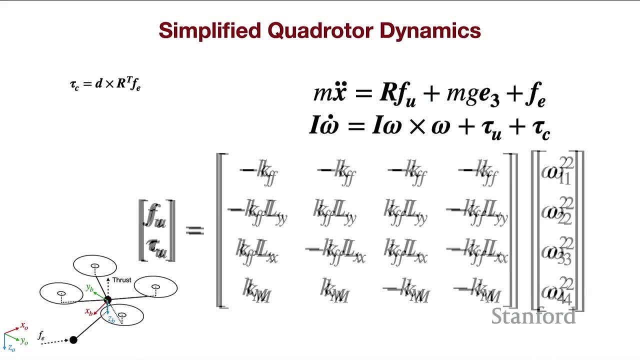 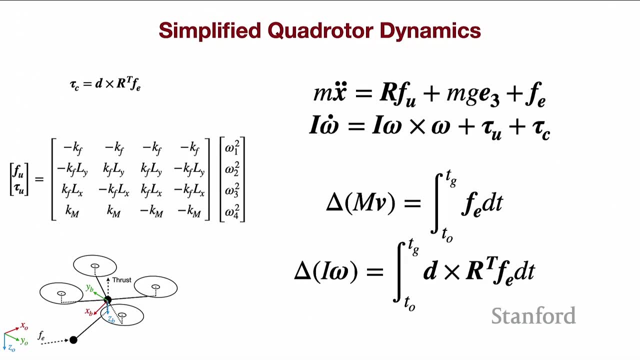 what you're controlling is the four rotors on the drone. Then, through this simplification, then we can say, okay, so this problem turned into the change in linear angular momentum resulted from this collision. So sure, now we have these equations. How do we make it? 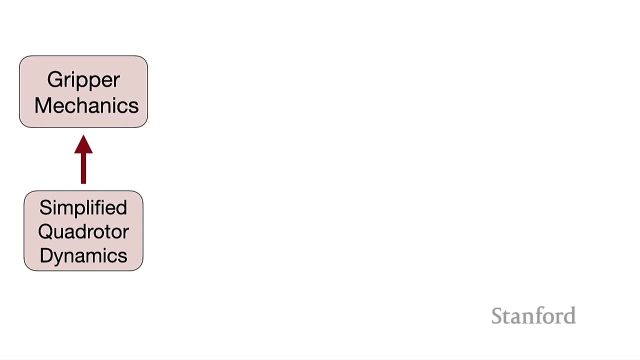 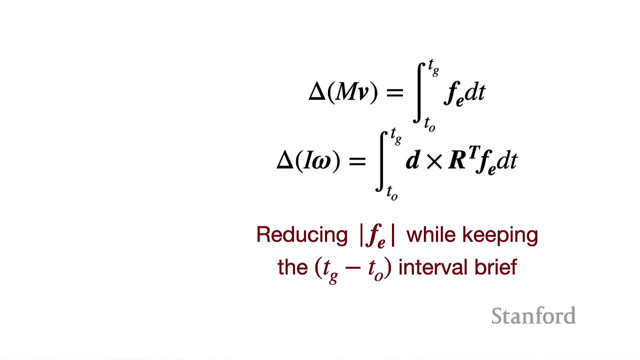 useful Because we're using these dynamics to inform our gripper mechanics. What does that mean? That means that from these two equations, what we can get, we want to reduce the magnitude of this force and reducing the interval as short as possible. More concretely, what does that mean for gripper design? Is that first one motivates a compliance. 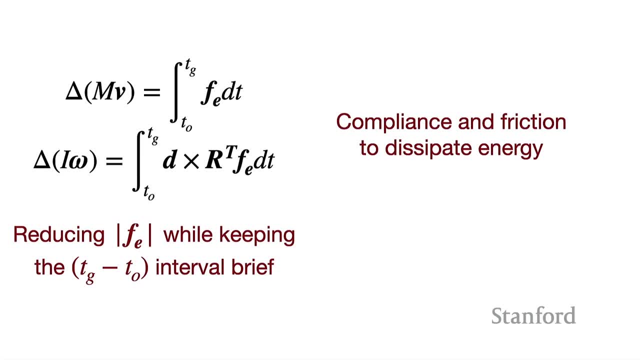 the use of compliance and friction to dissipate energy during the collision. And the second part motivates a fast-acting gripper. So the fast-acting gripper also has advantage of aerograsping, meaning that your target is now bouncing out of your grasp. So now we have these lessons. 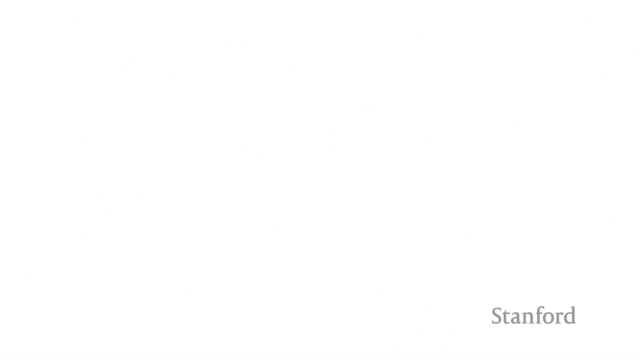 we're trying to design around And the three main goals we identify as the main point for this aerograsper is: one: we want to minimize the overall weight and inertia because the drone payload is very limited. Two: we want to maximize the allowable maximum velocity. 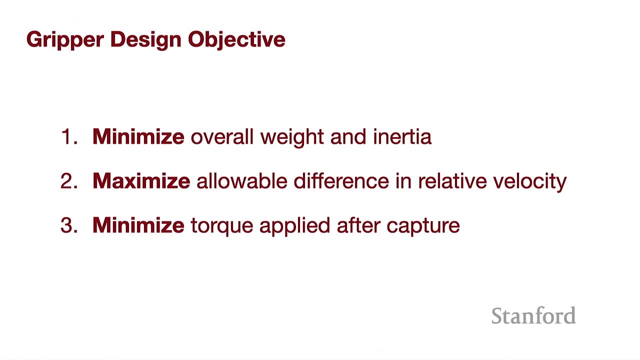 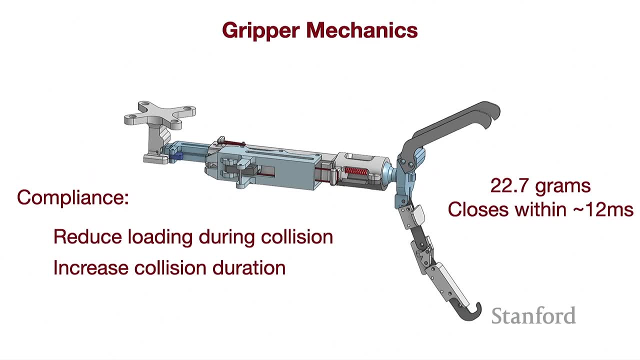 difference between the two drones And three. we want to minimize torque applied after the capture So the drone can remain safe even after the capture. So here's a gripper, a CAD of the gripper. We designed this gripper. It's all 3D printed. 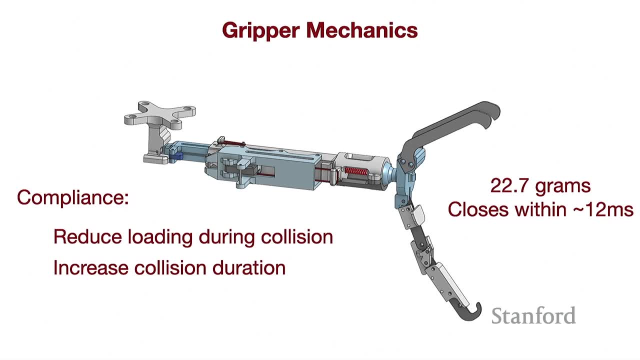 It weighs about 22.7 grams and can close within 12 milliseconds upon impact. We used a compliance suspension mechanism which to reduce the loading during collation and also increase the collation duration compared to a rigid gripper, And I have some videos later showing. 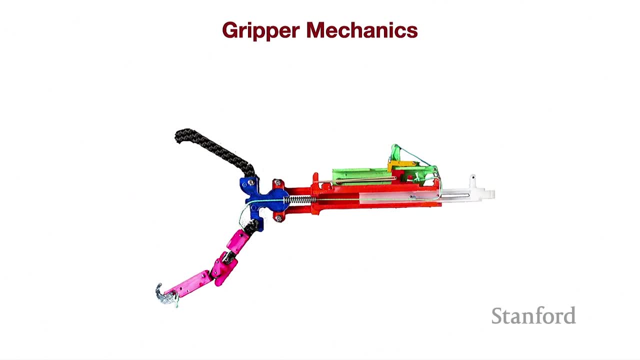 this. So how does the gripper work? Here's a cutaway of the gripper. You can see that the gripper. you have a force coming in from the collation And there's two parts of the gripper that slide. Oops, There's two parts of the gripper that slides on top of each other: The orange. 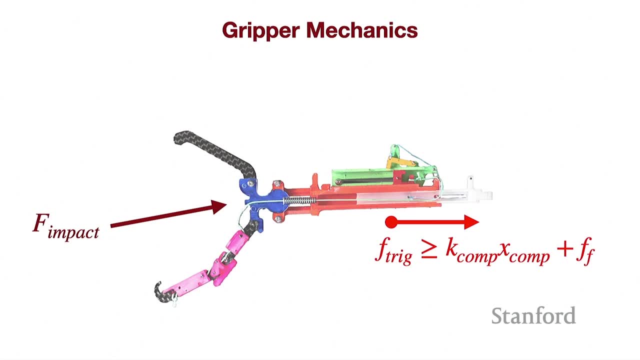 part and the white part, it slides backward. That's your linear compression, a linear compliance. And this relative movement between the two parts causes a blue tendon to pull the yellow trigger upwards and releases the red block which has rubber band in there to provide 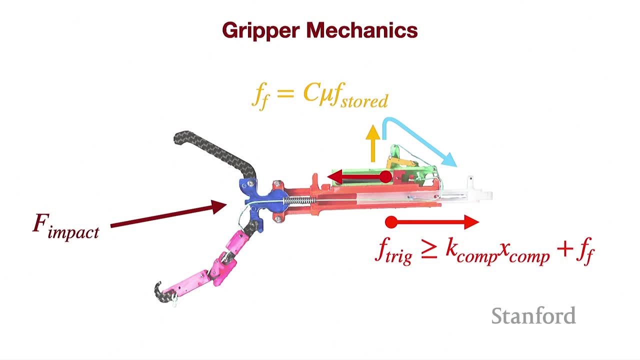 a potential energy. As soon as this trigger is pulled, the yellow trigger will be pulled. This red block accelerates forward and pulls this green tendon, which is connected through a bunch of tendon routing to the under-axiary finger on the bottom. Then it closes like. 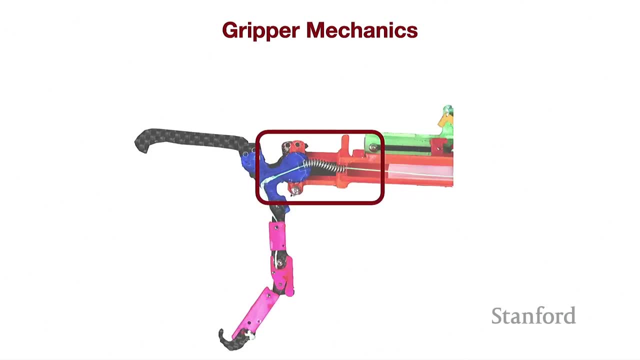 this And the blue part here you see is a self-centering ball joint where we built this, exploiting the nature of the torsional stiffness of a compression spring. This is very similar to for those of you who play games on your Joy-Con, on your controllers: how does your Joy-Sense 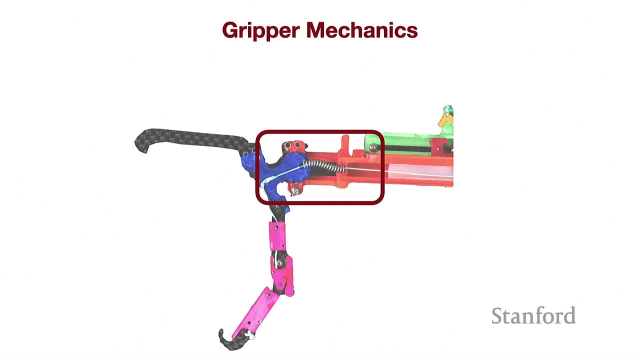 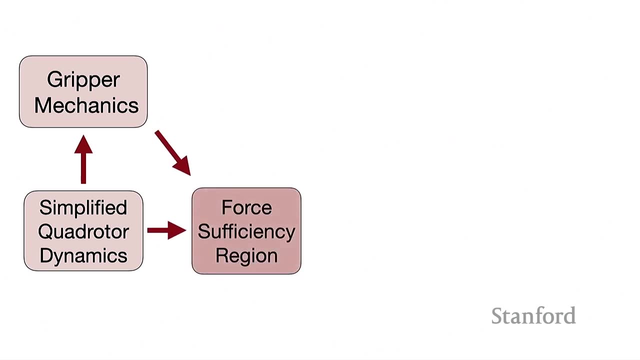 your joystick always self-centers after you apply input. Same principle here. So now, after understanding these things, what we want to move on to is what I call the force sufficiency region. We'll talk a little bit more about this. So we have this gripper. 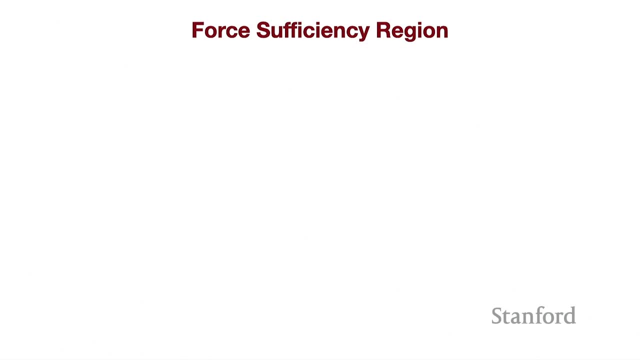 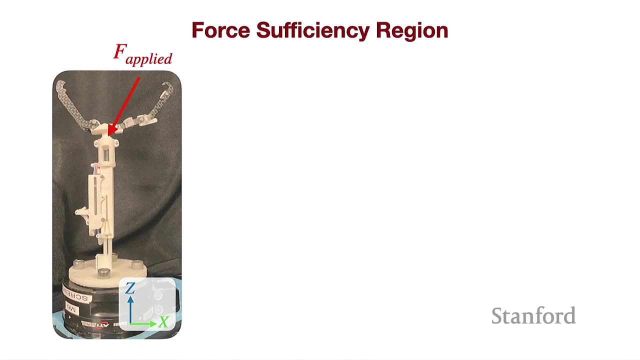 It's time to bring it into a bench top testing. How do we validate that it actually works? First, what we did was we mounted this on a six-axis force torque sensor ATI right here and we applied random force on the top. 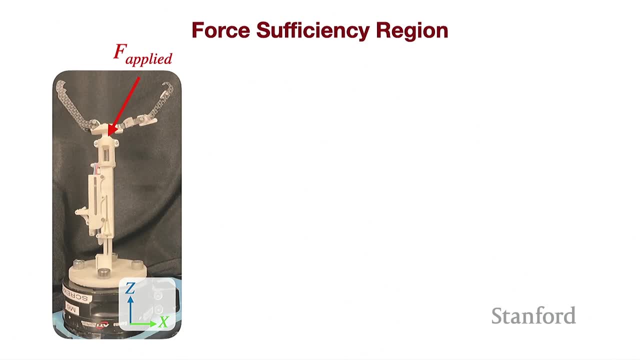 So we can see that empirically, after doing many, many, many trials, we can plot this in force space. It looks like this. So this limit surface in force space basically represents the minimum amount of force it needs from the collision to trigger the grasping sequence. 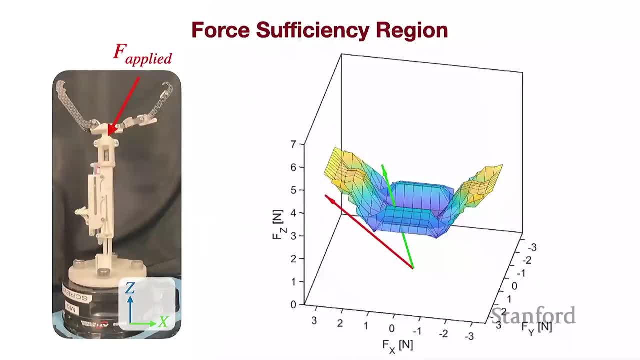 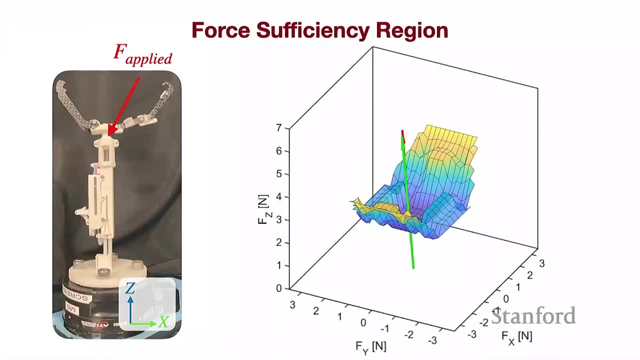 because everything is friction in there, And the two examples here is: the green vector pierces through this bottom limit surface. So then in this case the grasping sequence will trigger, And the red vector here does not never intersect with the surface. 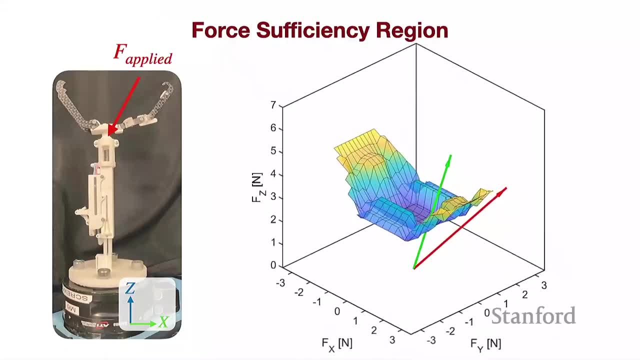 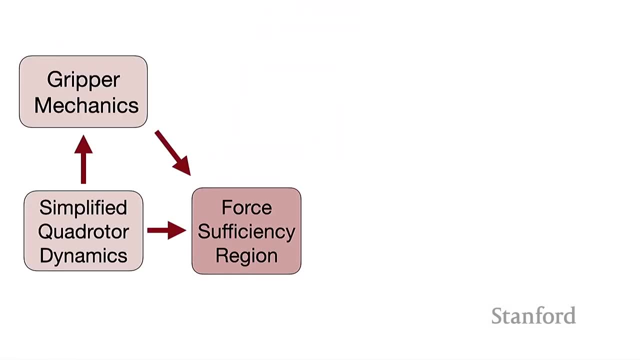 That means that force it's not going to be able to trigger a grasping sequence. So now, with this sort of force sufficiency region, I want to move over to velocity sufficiency region. Why do we need to do this? Because drones in nature is controlled by velocity. 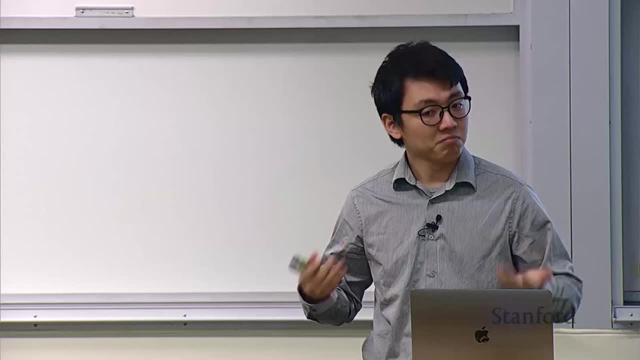 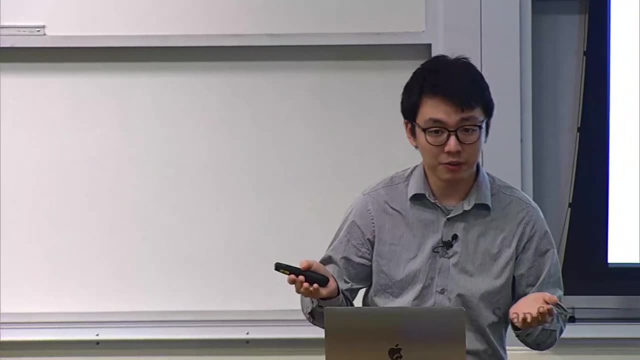 whether you give it position or velocity controlled, It's not too useful. you tell the drone: hey, can you hit the target at two newtons in this direction? Well, the drone doesn't know how to do that. It's like, OK, can you hit it at this particular velocity within this velocity envelope? Yeah, 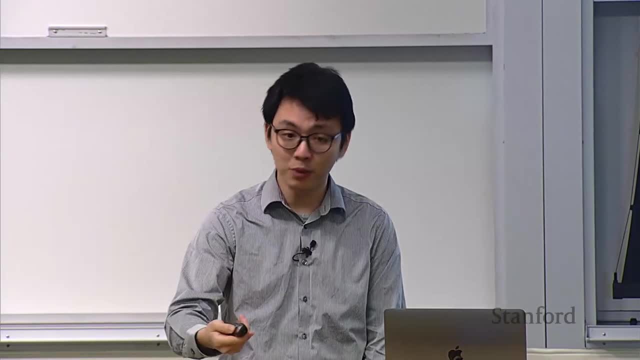 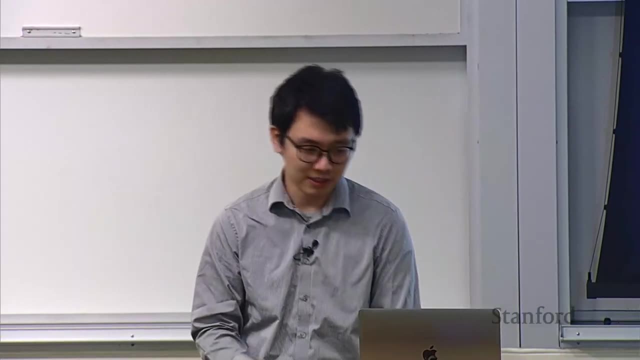 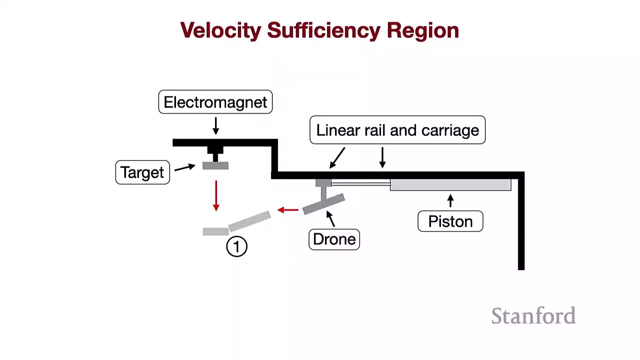 sure, There's plenty of algorithms out there right now that can compute a flat trajectory for you. So that's the importance of velocity sufficiency region. But then how do we go from force to velocity? Another experimental setup. So what we did here is we built an experimental setup: drones mounted on a linear rail powered by a pneumatic. 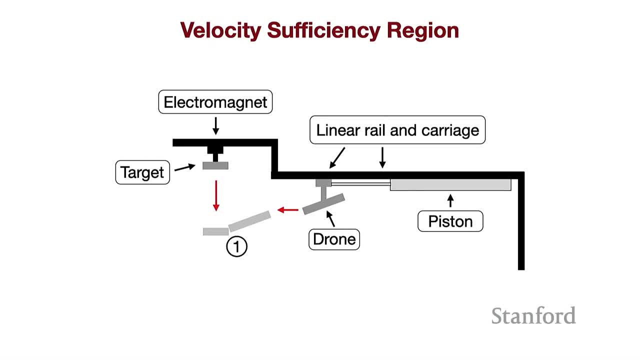 piston, So it actually launches the drone off the rail and hits the target drone at the exact moment, because it's controlled by an electromagnet. We have a force torque sensor mounted on the tip of the drone where the collision happens. You do this many times. 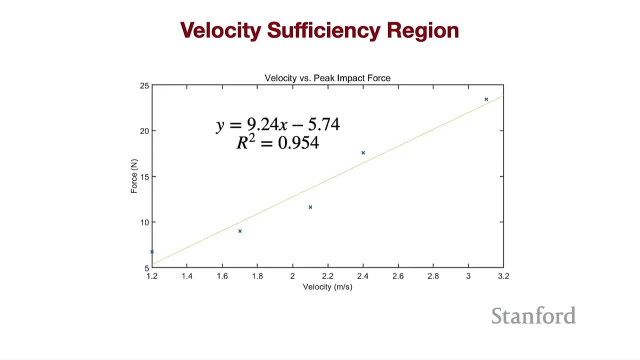 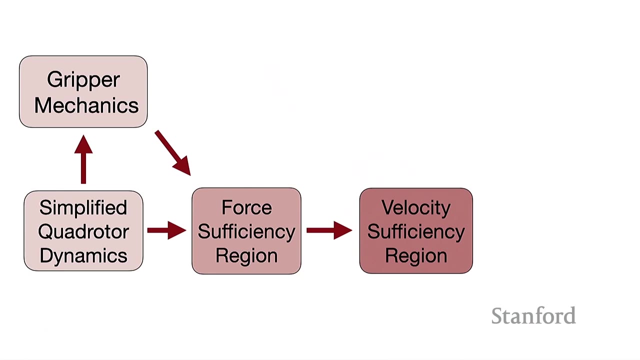 varying the pressure in the piston, which varies the velocity, gives you this linear relationship between velocity- the exit velocity of the main drone- and what's the peak impulse force we're experiencing at the point of collision. So with this, this can serve as a translator between force and velocity. space At this. 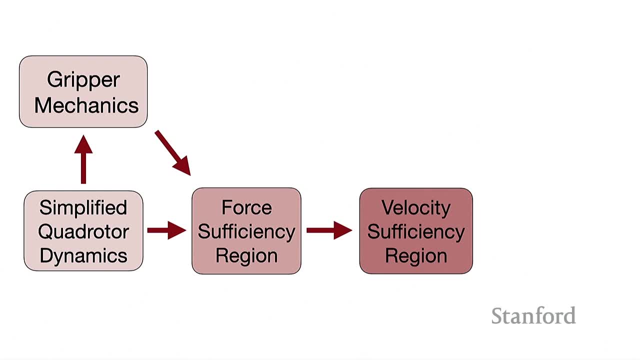 point. it's time to re-evaluate your data. So I'm going to go back to the design. Does the gripper at this point actually solve the problem? Does the gripper at this point actually meet the design requirement? If not, we have. 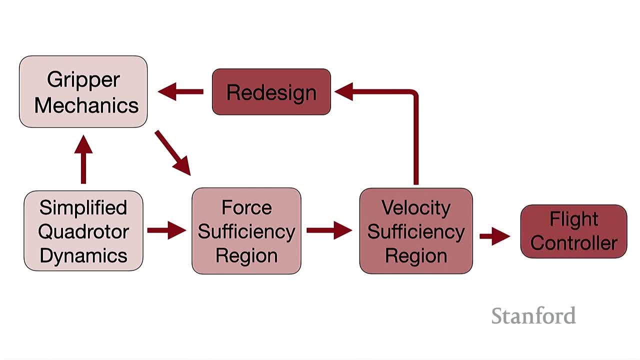 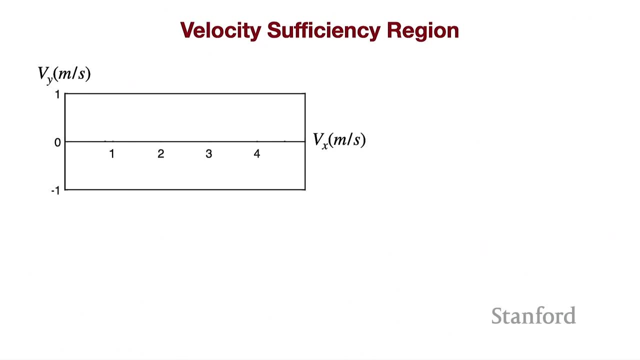 to go through a redesign process If it does time to go through the flight controller. So before I send you videos, I want to explain a little bit more about this velocity sufficiency region. So I'll redefine it here really quick. Basically it's a region in velocity space. 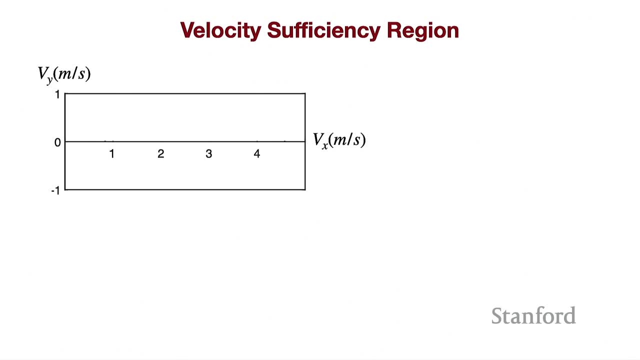 that is required to success. So I'll break this down a little bit more. Let's locate a 2D slide easier to do in 2D, in X and Y direction. The lower bound, basically, is determined from the force sufficiency region test. Basically, if your velocity is in that region, you don't. 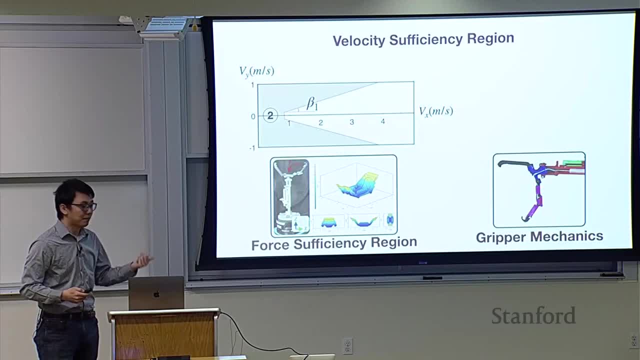 have enough force to trigger the grasping sequence. The sides are bounded by the gripper mechanics- how much compliance you have in the angular direction of the yaw and pitch direction of the gripper? And the sides and the top are bounded by the quadrider dynamics. 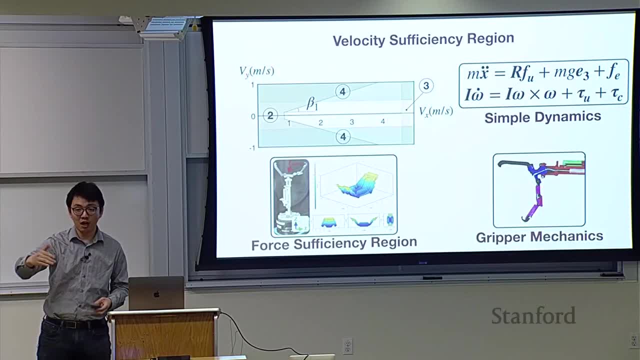 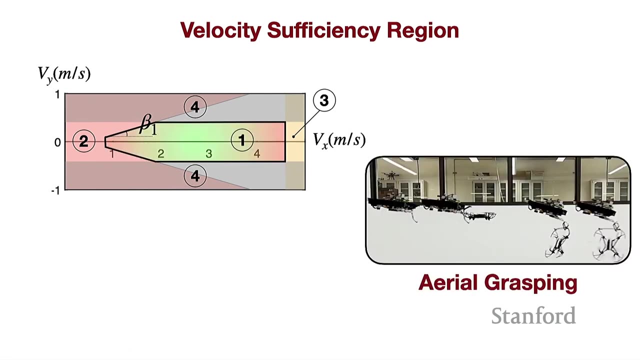 your quadrotor is running into another object in mid-flight, The resulting torque and force disturbance to the main drone needs to stay within the control authority. Your drone cannot crash after this intended collision. So this enclosed space right here is the velocity sufficiency region. 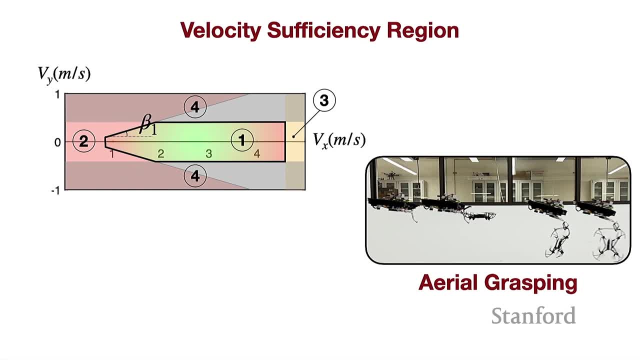 So basically, it's a combination of velocities that we can say: okay, the drone should try to hit a target with these velocity profiles to maximize the chances of success. The key point I want to point out here is that this region is not an absolute, but a gradient. 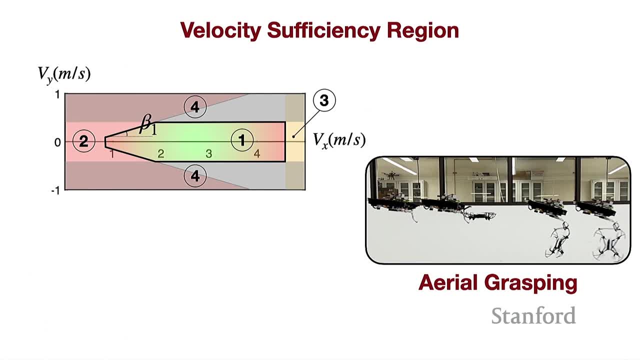 That means as your velocity conditions approach the boundary of this velocity region, the probability of success decreases. So there might be some failure. that happens even if your velocity is within this region and there might be some successes in there, even if it's outside this region. 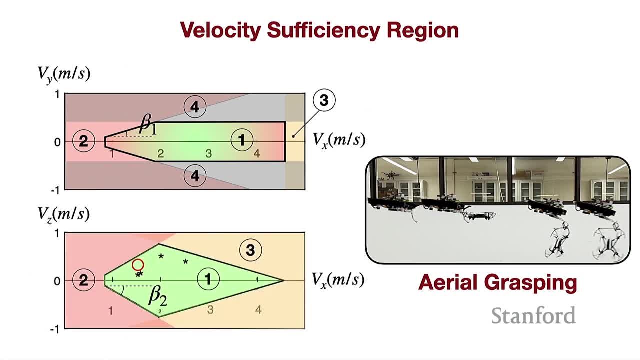 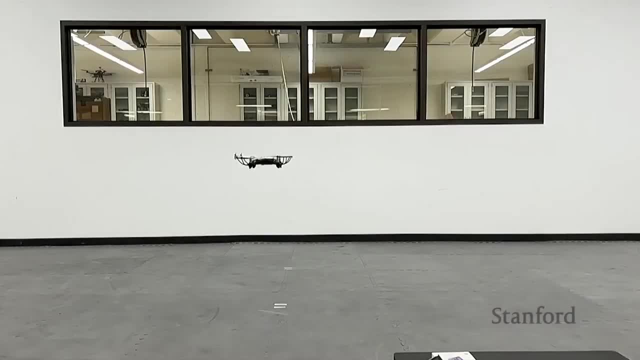 This is all probability-based. You can repeat the same thing to do for the XZ direction. Then it gives you the probability of success and it gives you this. So I'll explain a little bit more as the video is playing. So we're using a 500-gram drone with the gripper. 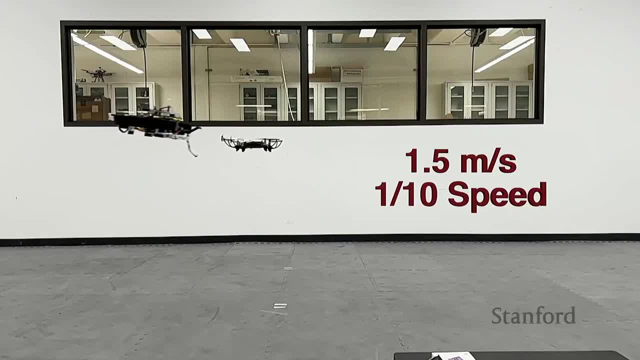 capturing about 85-gram modified mumble drone at various different velocities. Here is about 1.5 meters per second, played at 110 speed, and we repeat this many, many times. This is the fastest we have done is 2.7 meters per second. 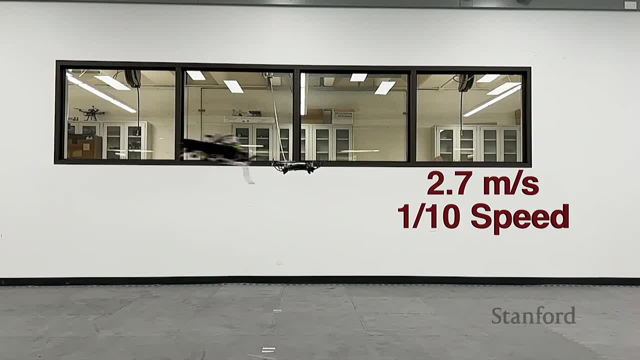 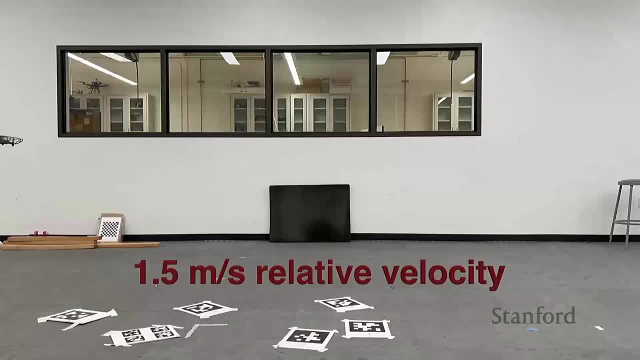 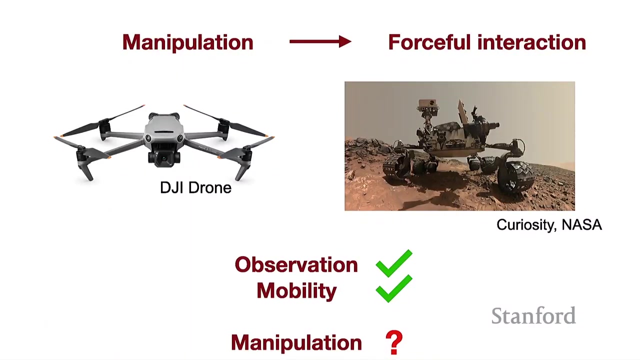 Yeah, the propeller didn't make it, So this is capturing at relative velocity, basically moving targets. OK, so this is for area grasping. This is what we did and why we did it, So I want to move on to the second part of this talk. 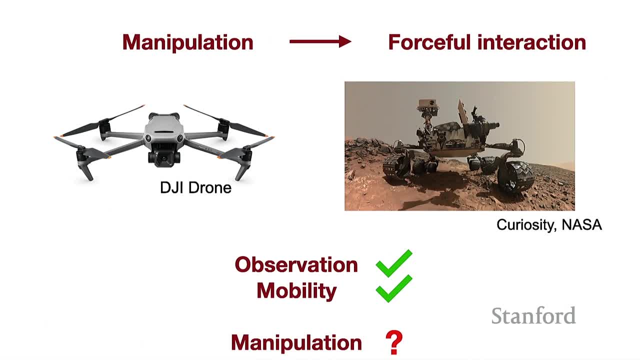 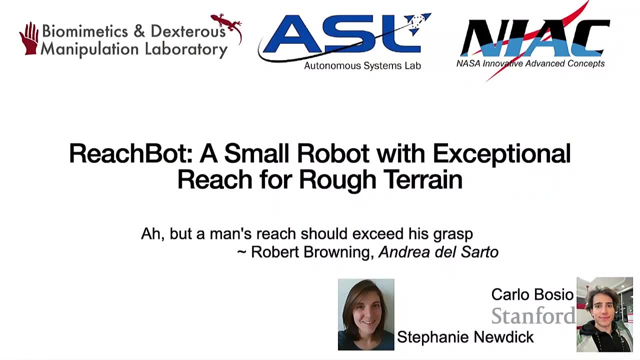 Let's talk about planetary exploration. So here I have a picture of the community. This is a very small robot. It is a small robot. It's an aircraft carrier. It's a small robot. It's on a plane. It's a pilot. 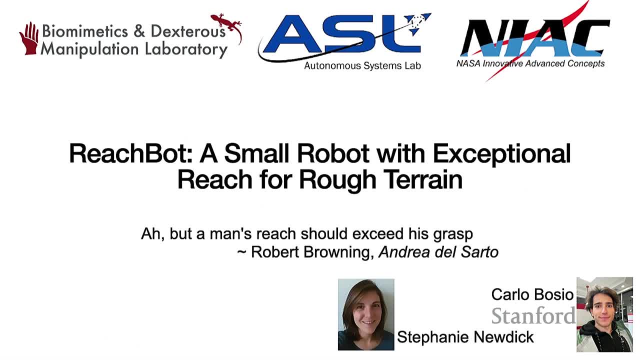 It's a helicopter. It's a helicopter And our robot is called Reach Bot and it's a small robot with exceptional reach for rough terrain, And this is a collaboration between our lab BDML and ASL over at AeroAstro and collaborators Stephanie. 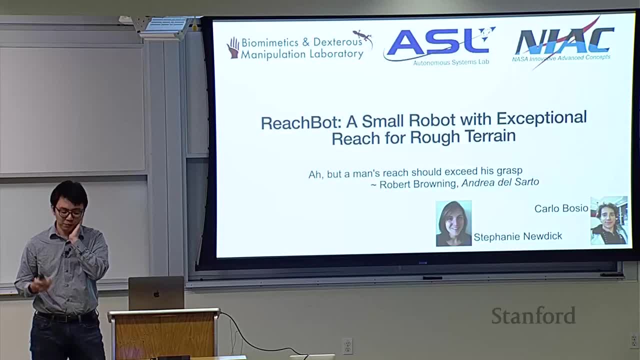 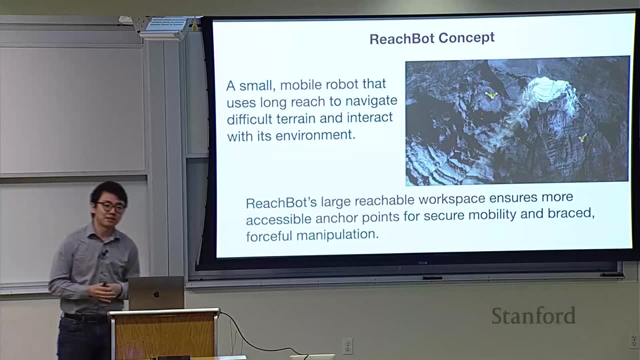 who's a student in ASL, and Carlo, who was an exchange student in our lab and now he's a PhD student at Berkeley. So what is Reach Bot? The concept is this: It's a robot that connects to the ground. 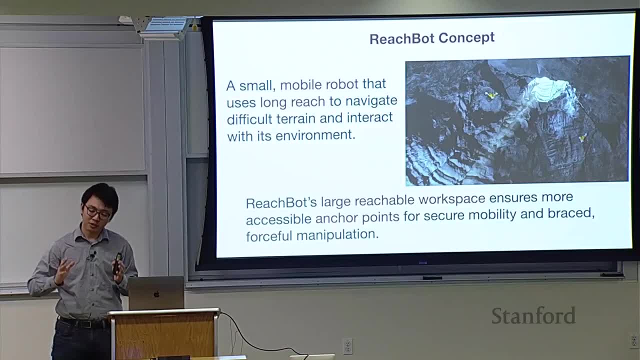 a small mobile robot that uses long reach to navigate really difficult terrains and interact with the environment. It has a really really large workspace, ensures more accessible grasping spots and faster traverse across certain areas. So what's the problem? here? You see a state-of-the-art climbing robot. 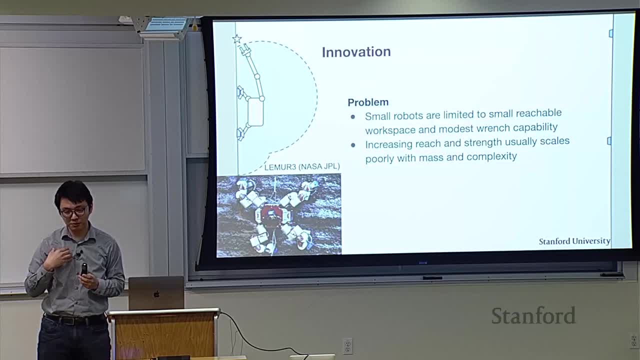 Here's the Lemur 3. here you see on the bottom. Just like you and me also, when we go to the climbing wall, I always feel like I could use a longer arm. Once I'm on the wall, can I reach the next hold? 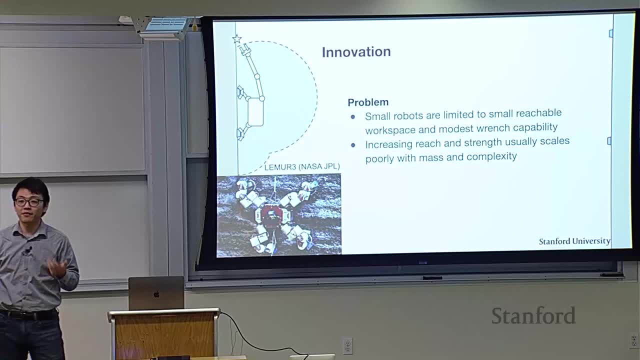 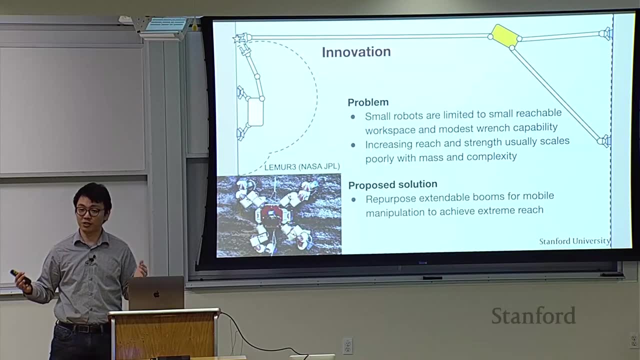 It's limited by the length of my arm. But what now? What if your arm is actually extendable like this? Now that suddenly you have a lot larger workspace you can search, You might not run into dead spots where you thought that you could get to the target. 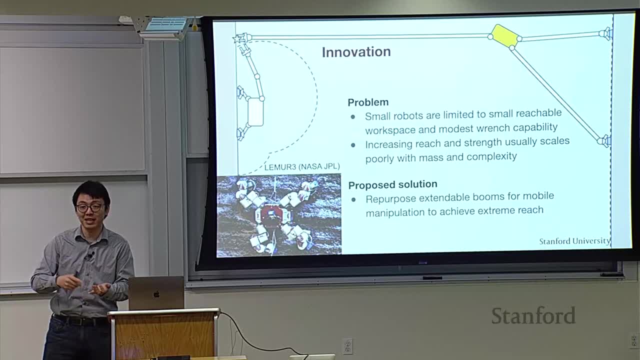 but suddenly in certain parts midway through the trajectory, you realize you can't reach the next grasping spot. So this is our proposed solution: We use repurposed extendable booms for mobile manipulation to achieve extreme reach. The enabling technology here is these space booms. 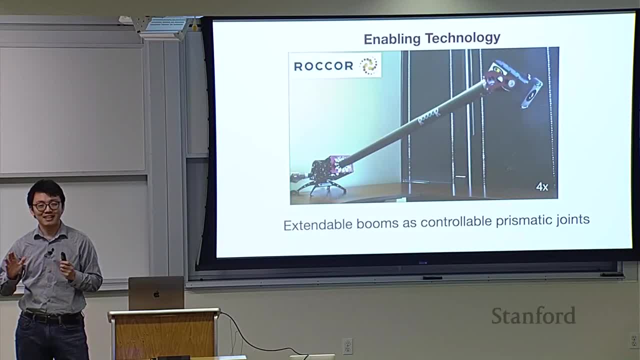 They collapse really. Just imagine them as 3D tape measures- And this is actually a thing built by Rokor used to deploy a camera in space outside the space station. They compact really small and then they fold out in a 3D thing, just exactly like a 3D tape. 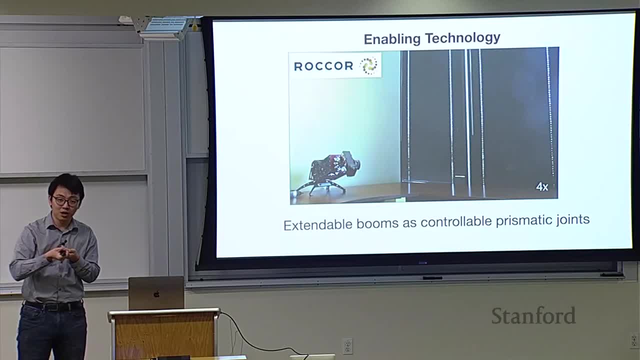 measure. They're really strong in tension so you can pull on them as hard as you can, just like a tape measure. But with any other force conditions they're easily buckable, So they can go through buckle fairly easily. So these are the extendable booms we're. 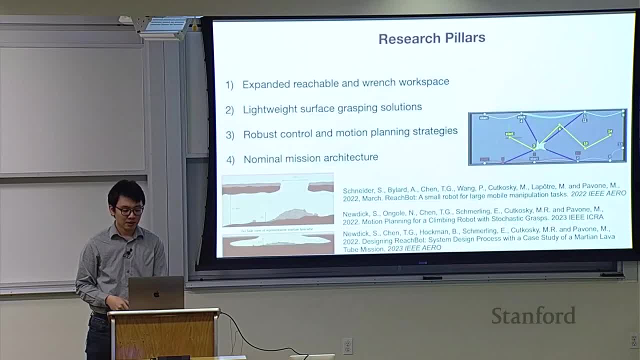 proposing to use as arms. So we have a lot of research pillar. This is a brand new concept we're trying to propose. There's a lot of things we need to investigate And my colleague, Stephanie, mainly focuses on trajectory planning and the trajectory optimization of this. 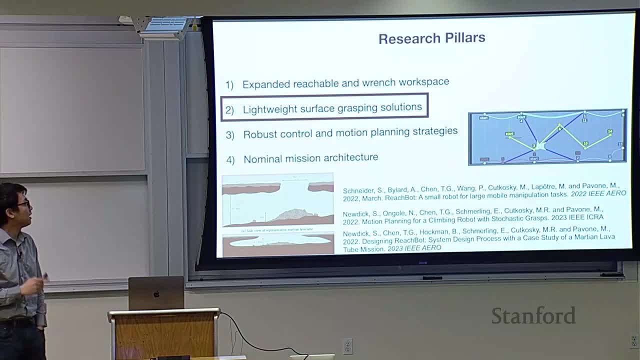 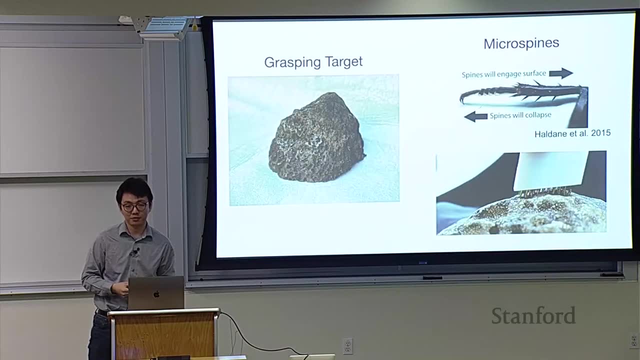 But today I want to mostly focus on two here: Lightweight surface grasping solutions. So if we're talking about grasping solutions, the first thing is: what are we trying to grasp? A lot of this lava under the NASA grant. 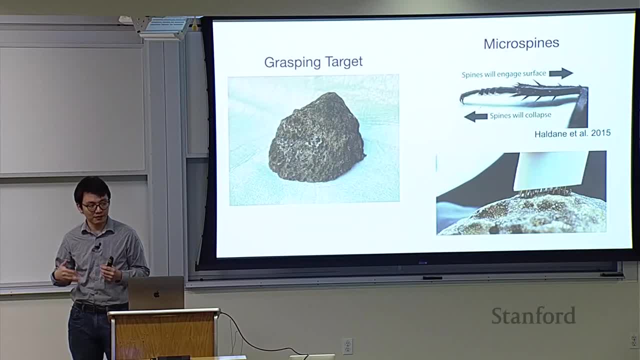 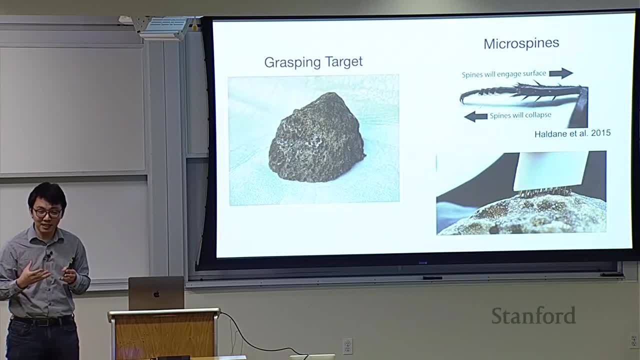 very, very good, And the reason why it's so inspired is inspired from insects such as cockroaches. Unfortunately, cockroaches are really really good at climbing vertical walls, And the reason why they can do that is that they have these hard spines at their legs. 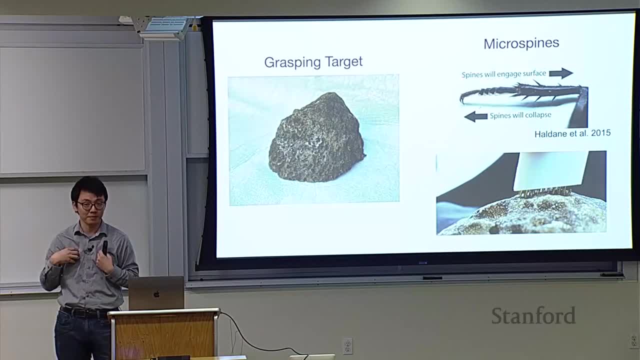 It catches on the small asperities onto seemingly smooth walls to you and me, But it's enough to give them the adhesion they need to climb a lot of the surfaces that we think is smooth. With the same principle, we use these almost needles. 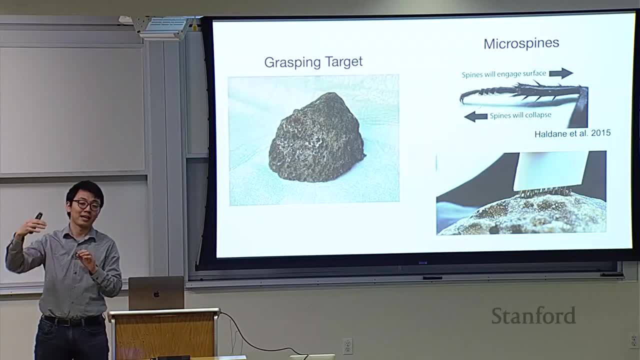 on the bottom. here you see that it uses the same principle that caches on these small asperities on rock surfaces to give us adhesion. So this is just a quick overview of the technology we're using. We have this entire new concept Of 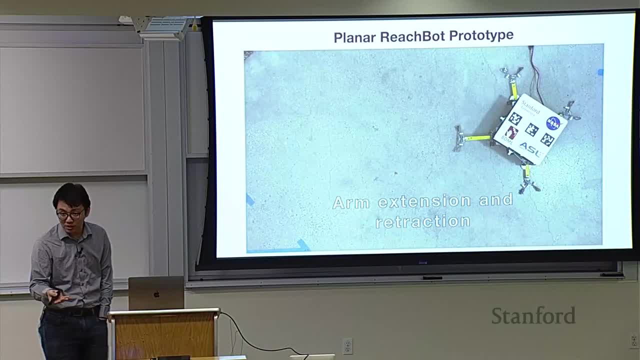 course we're not just gonna go out there. we don't have the money either, or the time, or we don't even know if this thing's gonna work to build a whole system, So we need to start somewhere. So what we start is to build a planar. 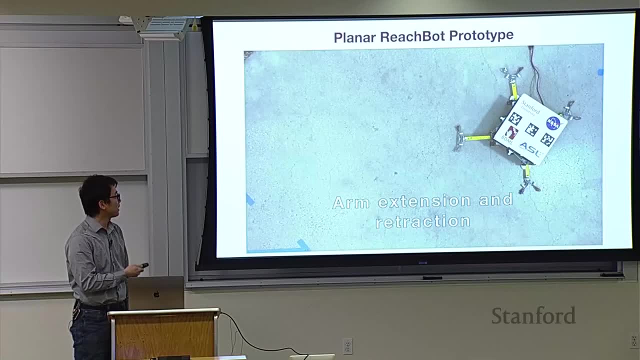 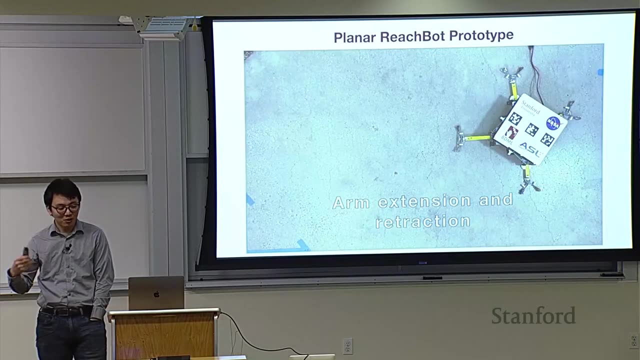 prototype, low-cost planar prototype. You see, here's a planar reach bot that rolls on four bearings, that's free floating on a flat surface And, like I was hinting earlier, what's the 2D, cheap alternative to these expensive space. 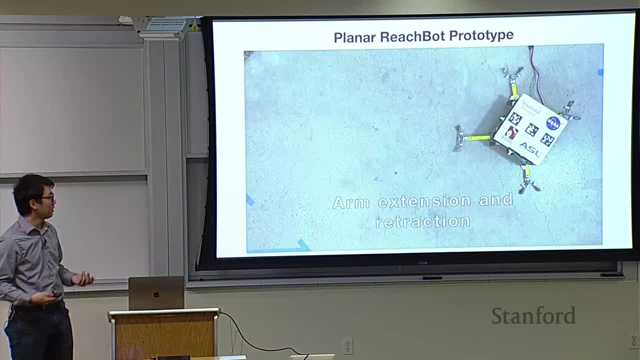 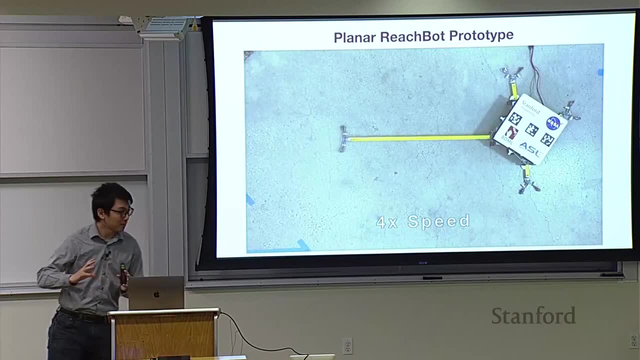 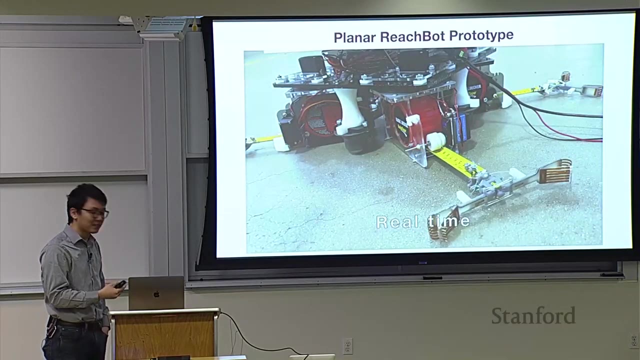 booms Tape measure, So we motorize these tape measure to extend and retract. And each of these tape measure unit arm is mounted on a servo so that it can rotate, pivot the shoulder joint as well. So it does all the basic functionality of proof-of-concept for a reach bot. 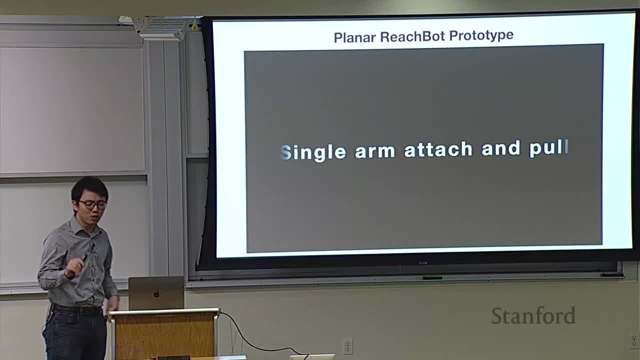 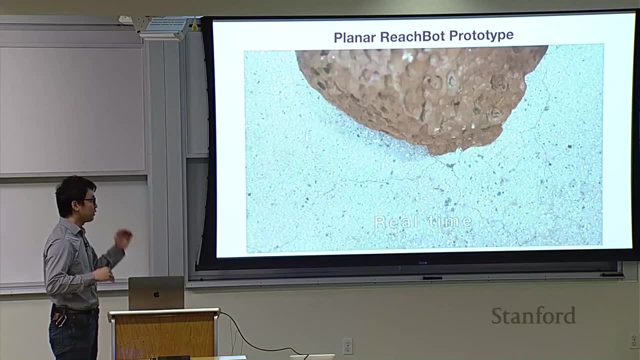 It has this micro-respirant gripper, which I'll go in slightly more detail after this. I want to show the sequence really quick. It extends out, it identifies a grasping spot, it extends out, it uses a passively triggered gripper. So all you. 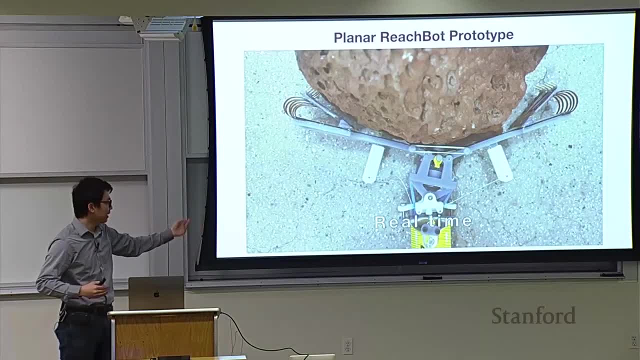 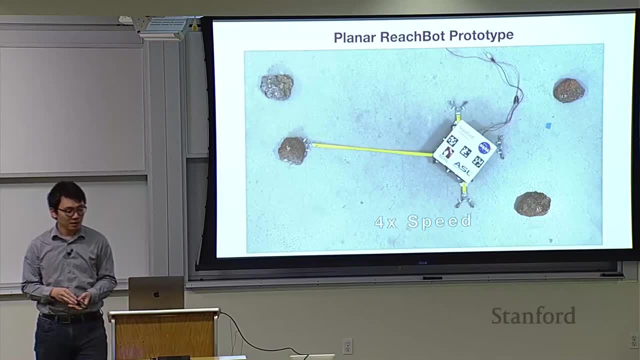 have to do is ram it into it. it triggers, it store the energy and then you can pull on it really quick to give you this adhesion. So now you can move your robot to that location. So this is one of the first tests we did with ReachBot, or playing on ReachBot. 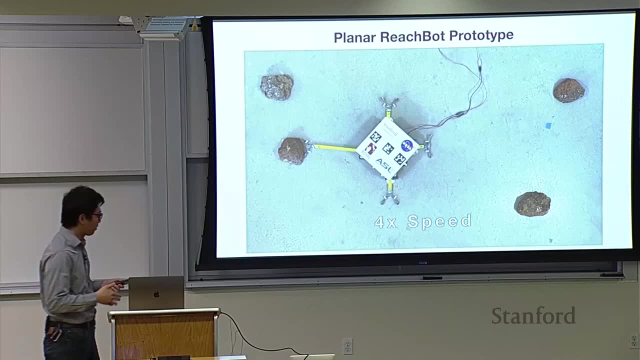 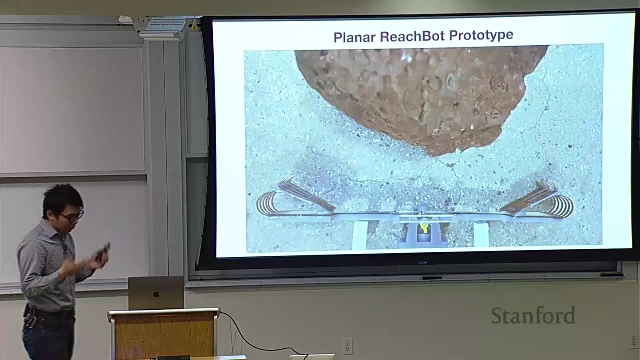 And now, with this capability, you can do a lot more interesting things, such as: now you have a free floating robot And the gripper resets, And you can do a lot more interesting things. You have a free floating platform that you can just move around, But now, with these grippers, you can actually anchor. 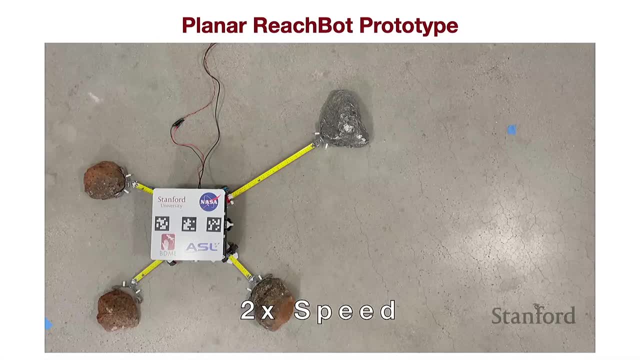 yourself to the environment. And now you're able to move an object that's way heavier than previously. what you're able to do- And this is callederen Isaac- We can just week that object. togethertam is a simple demonstration of that. And now you manipulate to a target location that you want. 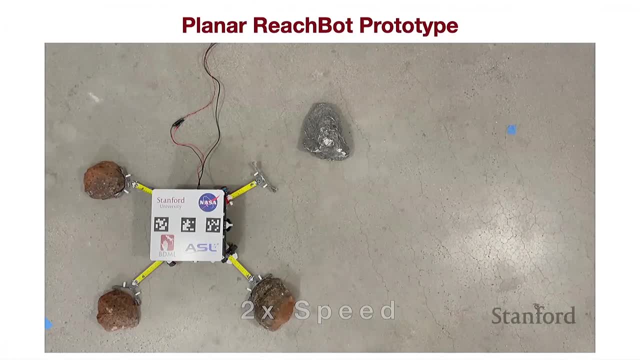 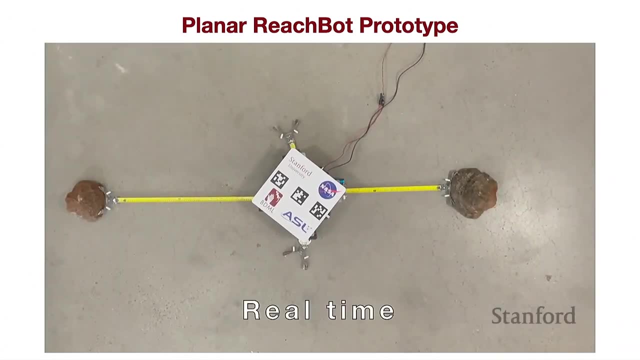 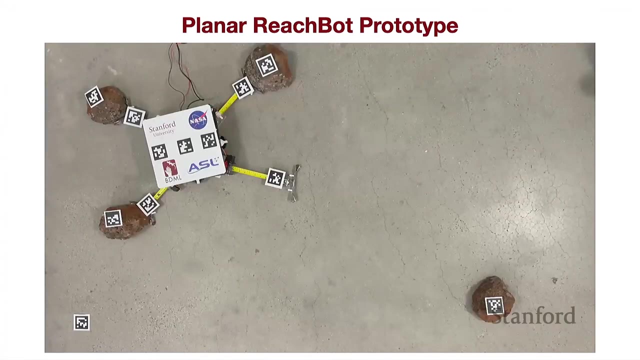 OK, we can let that go And we can do. how does robot move? This is a very simple case scenario where, as long as you maintain tension inside of your arms, you can translate between multiple anchor points like this, So the whole system will look like this: 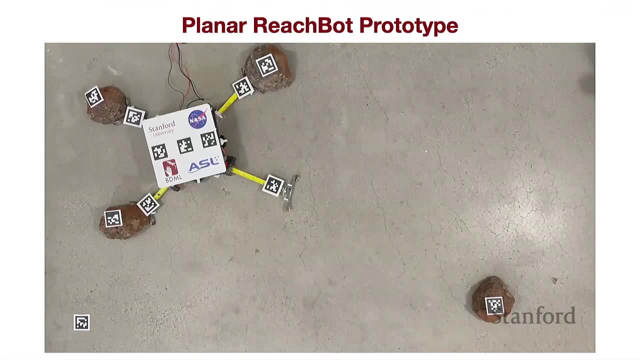 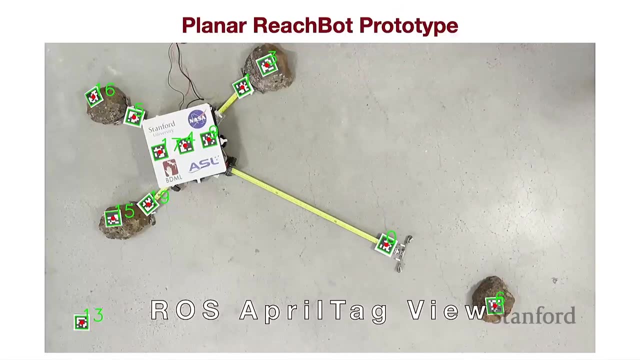 This is a demonstration we put together. is that you are anchored into a certain spot and you are scanning around. You are looking for the next grasping spot. You identify this as a potential grasping spot. You extend your arm out, touches it. it activates a grip. 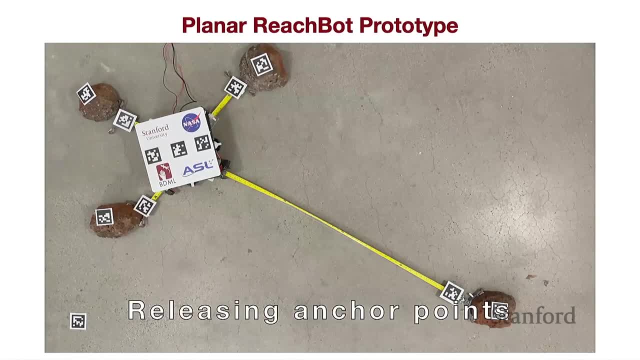 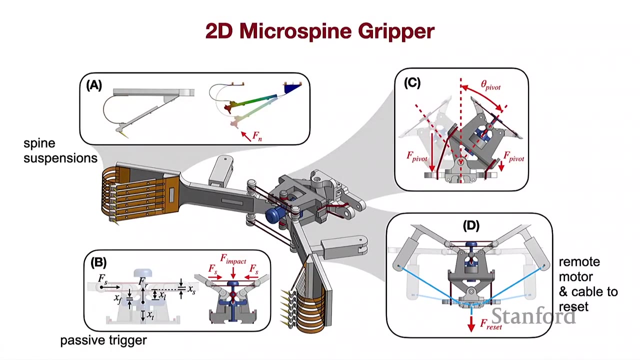 confirms that it's there, it's attached, And then you release and you pull yourself towards the target. So the 2D gripper here. so this whole robot was built as a proof of concept. It was built to convince ourselves and other people. 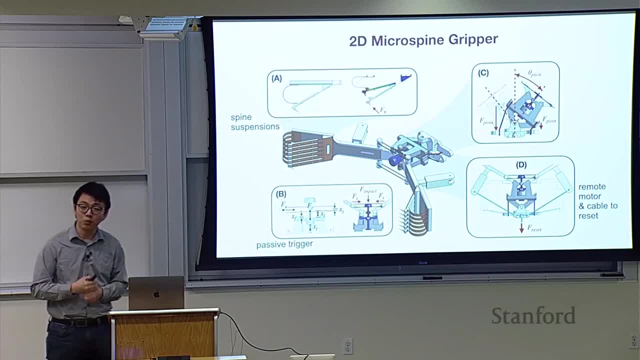 that this concept works. So for the gripper, we just need something quick and dirty that it works. So we have these microspine grippers on individual suspensions and we have a passively triggered gripper. Here we use a passively triggered gripper. 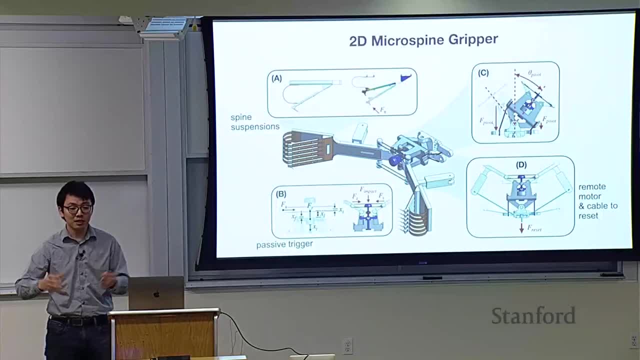 because we really need to minimize the amount of weight we put at the end of the boom. Normally it doesn't seem too much weight, but as you increase the weight at the boom and they extend all the way out, maybe four, three, four. 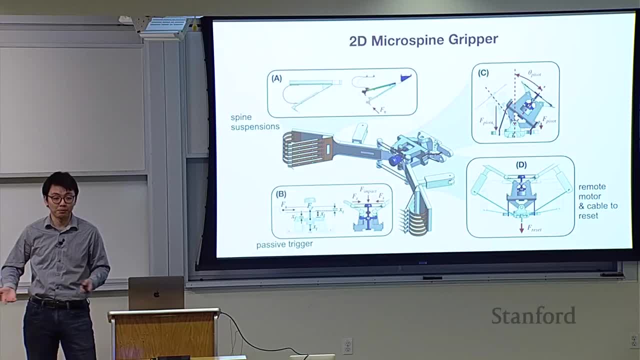 five meters. then it becomes a huge weight, inertia. you are swinging around And it can buckle your boom easily. So we had to really minimize the weight. But we just built something that works. But now we're trying to convince ourselves this thing works. then we need to move into 3D. 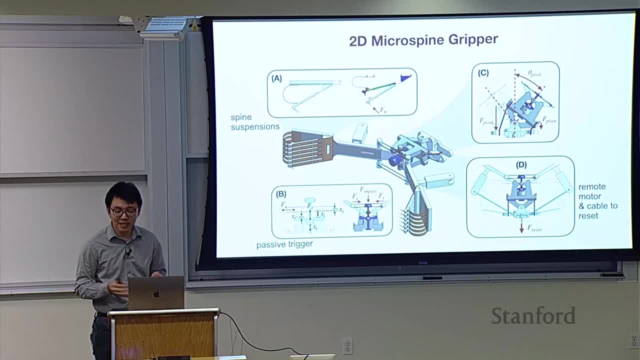 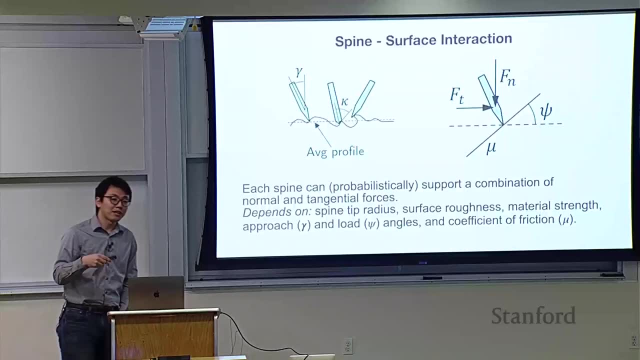 How do we actually build a 3D gripper? So it's with the same train of thought that I talked about before. Where do we have to start? We had to start with modeling. So first we had to understand the spine-surface interaction. 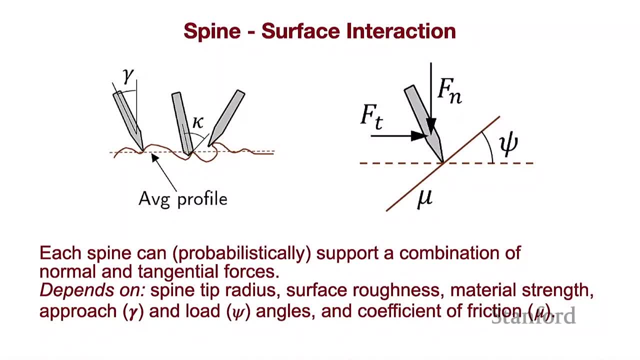 There are a lot that goes on here, Because the rock surface is stochastic, so everything is probability-based. So all of these, All of these forces are dependent on a lot of things like spine-tip radius, surface roughness, material strength. 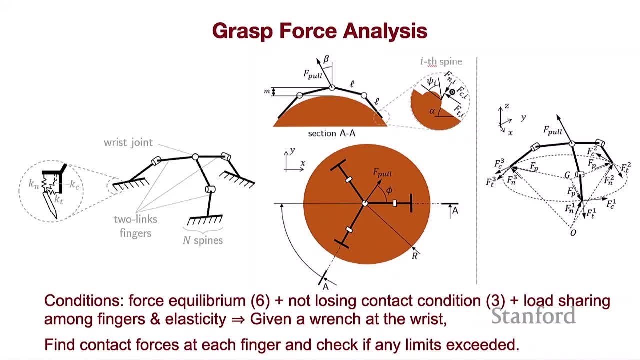 a lot of these things. Once we understand the surface- and this is ongoing research- So once we understand the surface and spine-surface interaction, then we say, OK, let's go with a three-finger gripper. Now you can write all your kinematics of it. 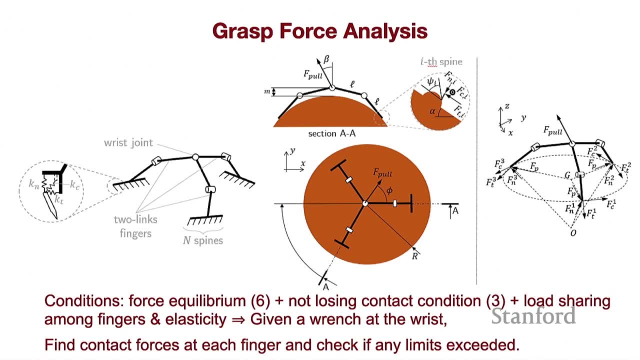 try to come with force, equilibrium and contact conditions, try to write equations for the whole entire surface, and then you can use a four-finger gripper for dynamic statics and dynamics And after all this it can give you, basically a wrench that you can apply at the wrist. 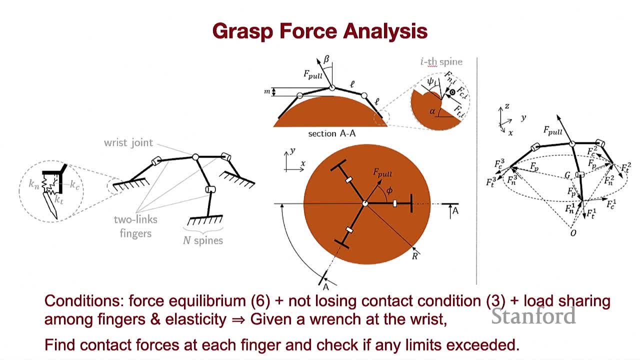 So that's the thing we're after. It's basically how strong are these grippers attached to the rock and how hard we can pull on things. And you can go through. since everything is probabilistic, you can go through a multi-column simulation. 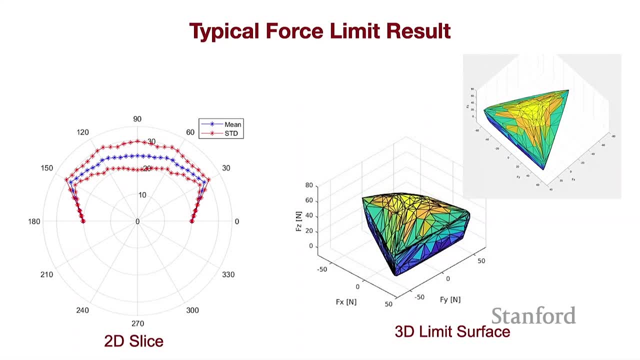 and it gives you something like this: a force limit. So it gives you a force, It gives you a limit surface in force space. basically saying, given the parameters of the gripper, how much force can you reasonably get out of the gripper once it's firmly attached to a surface? 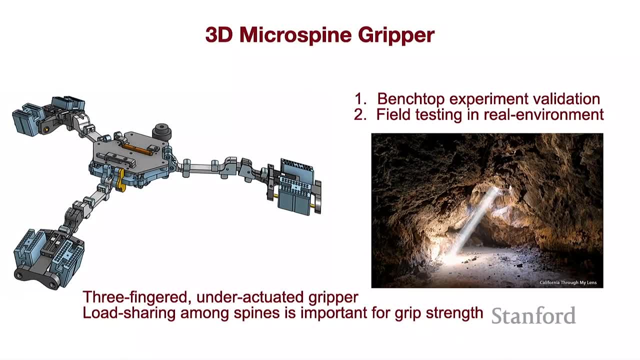 Once we have the model, we go ahead and build the gripper, And we're still working through multiple iterations and working on all the kinks of it. Once we have a gripper, what do we do next? So we haven't done this yet, but this is the next step. 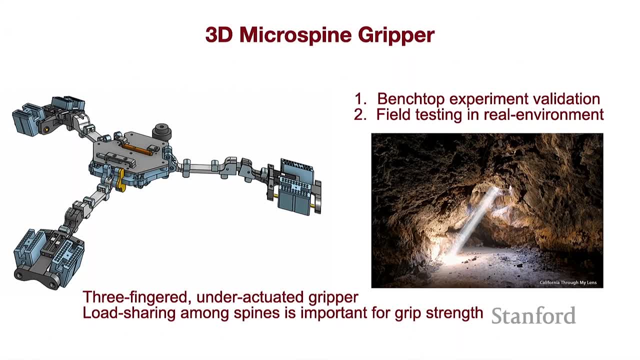 is, while we have a model, we have a prototype, the same flow logic. Then we have to test it in a lab setting environment. We have to do a bunch of lab tests, pool tests on it and try to make sure that it can achieve the desired grasping. 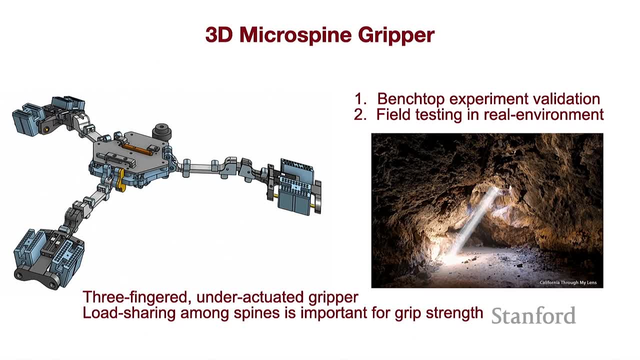 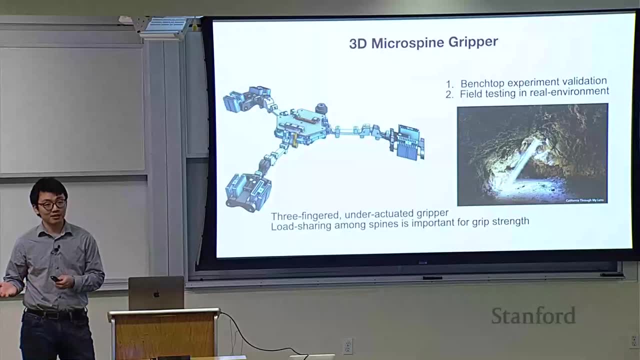 that force that we want. After that, after we validate the model, we either have to go through a redesign process and make sure that we hit the target, the design requirement, Or if it's good enough, then let's go test in the field. 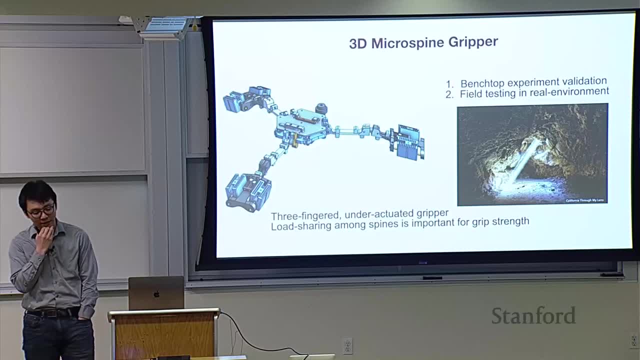 So right now we're scoping out. This is a lava tube actually at Mojave Desert that we're going to go later this quarter try to scope out and build a partial reach bar there so that we can show the whole. 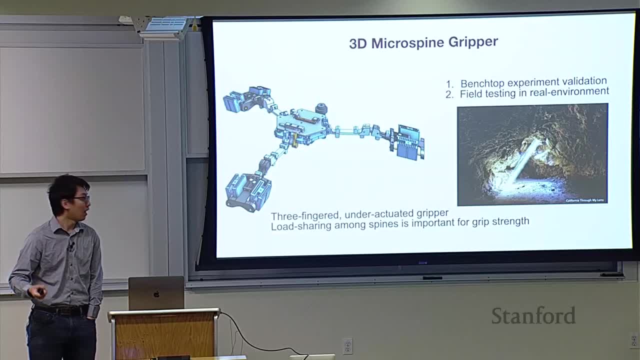 The whole system working of scanning the area, try to grasp part of the rock, try to pull on it to a certain degree and see to validate our model. So that's why we're here and I think that's the last slide I have. 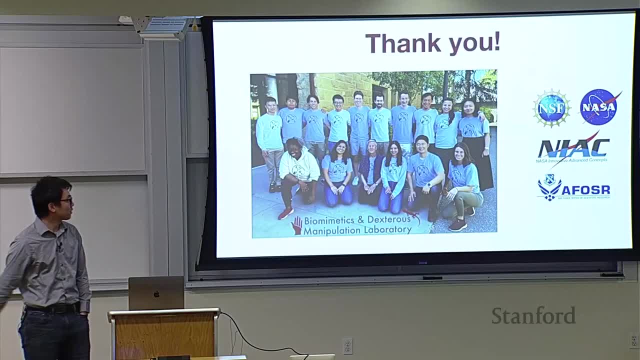 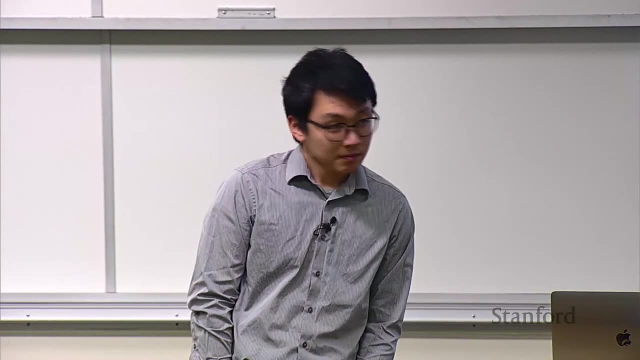 And I just want to say thank you really quick from the lab and all the funding sources supporting this project And I think I'll take questions. I think that's about 21 minutes. I'll take some questions, Yeah. So first of all, it's very impressive. 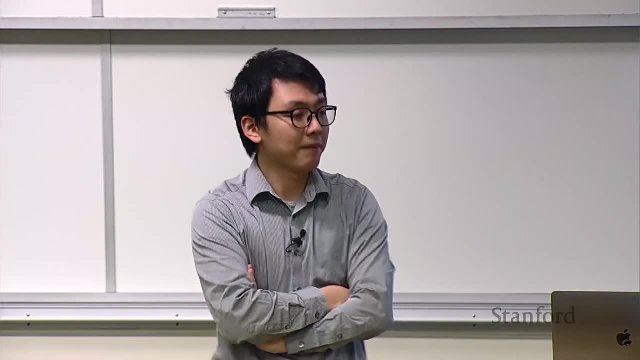 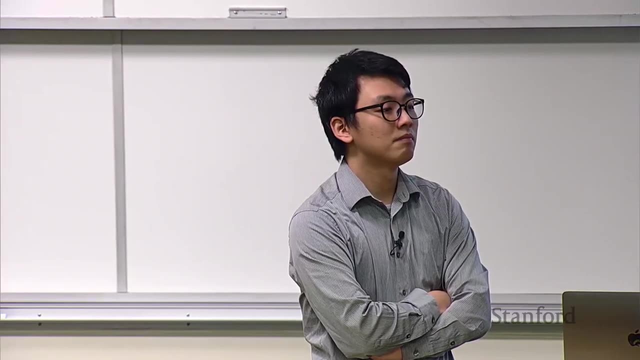 So you said this robot's purpose was for exploring And I'm wondering: based off of the movement, and how fast can it go? what's the reasonable estimate to how much area you think this robot can explore? It just seems quite slow, Yeah. 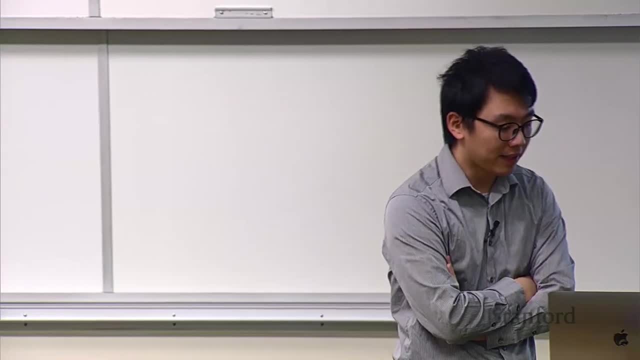 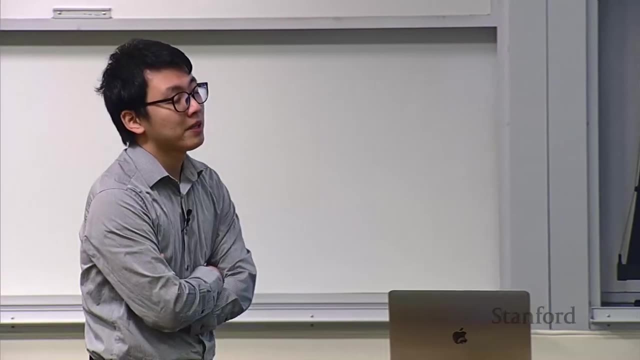 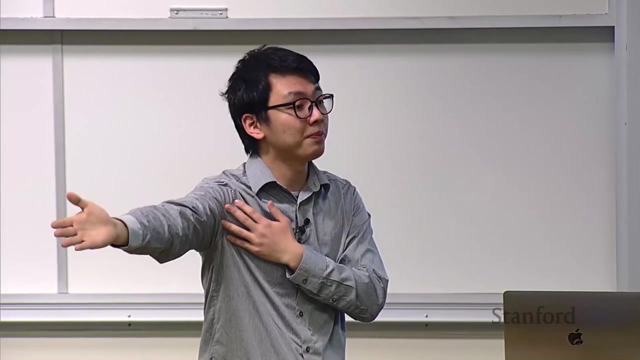 So that's a good question. So I think it depends A lot of things. the current scenario we're looking at is Martian. You know You look at different like planetary gravity means that how heavy does your robot to be? How long can you extend the boom before it buckles? 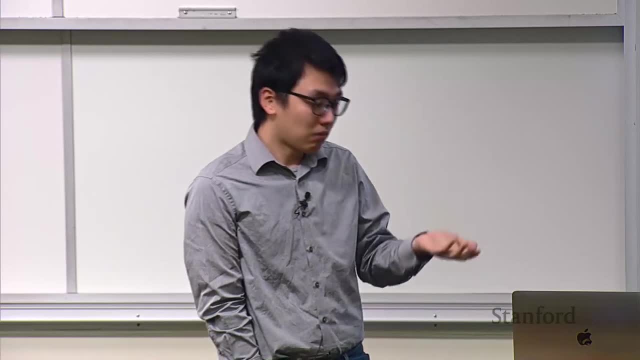 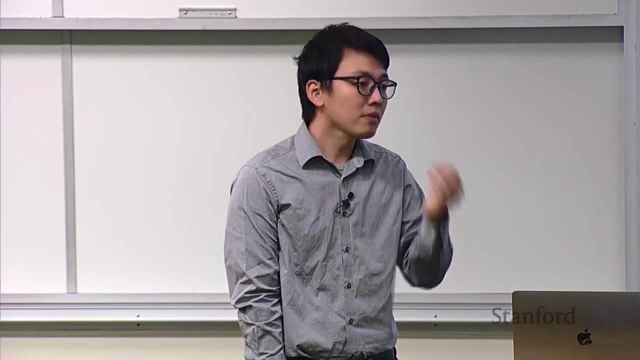 So it really depends on what gravity region you were talking about here. A good thing about NASA is that when you talk about these planetary explorations, they don't really care how fast you go And you compare it to the baseline of what we're comparing right now: a rigid link robot. 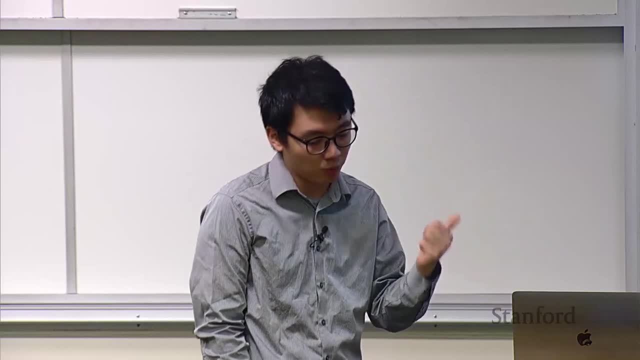 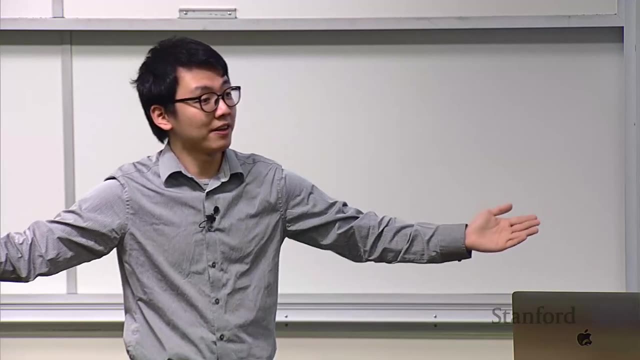 It should be able to one. it has two distinct advantages. One is that it can reach a lot more grasping spot at a certain point. Two, to go from one side of the room to the other, if my leg is twice as long I need. 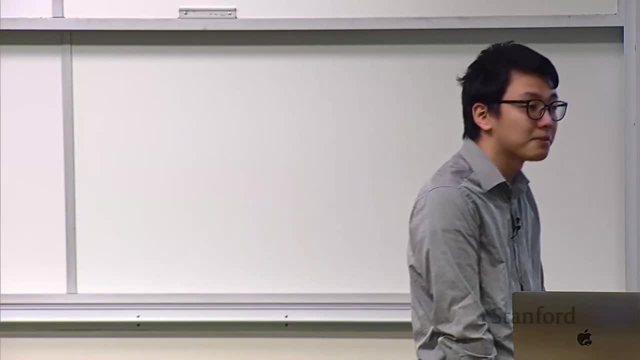 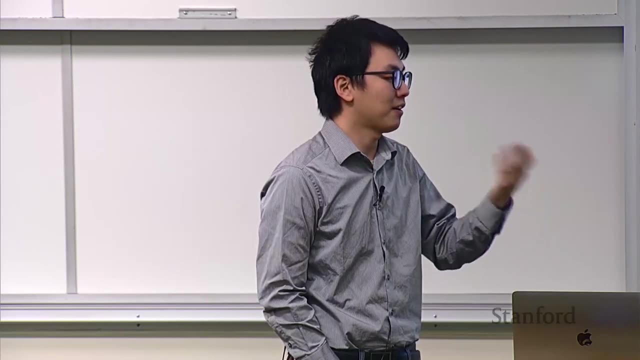 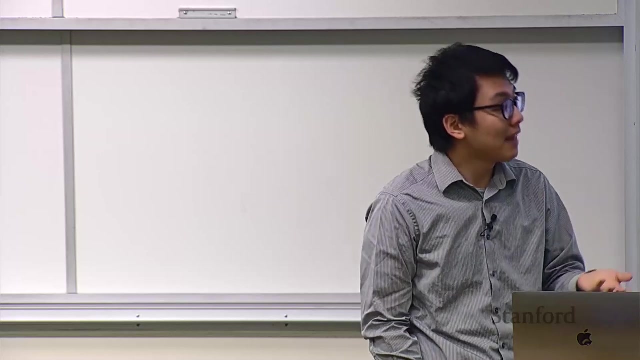 to take twice as little steps, twice fewer steps from one room to another. So we get that working for us as well. But if you're talking about another application we're thinking about ReachBot is for space station servicing, But then that actually becomes easier. 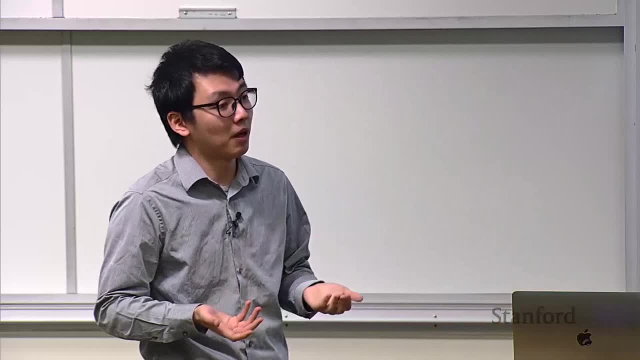 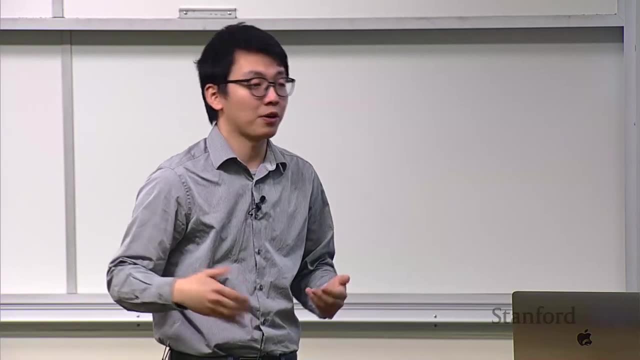 because that's in microgravity. Then you don't reach it. You don't really have to worry about part of the gravity, your boom, extending out nearly as much, the whole thing buckling So that you have even a longer reach. then you might be able to go from point A to point B. 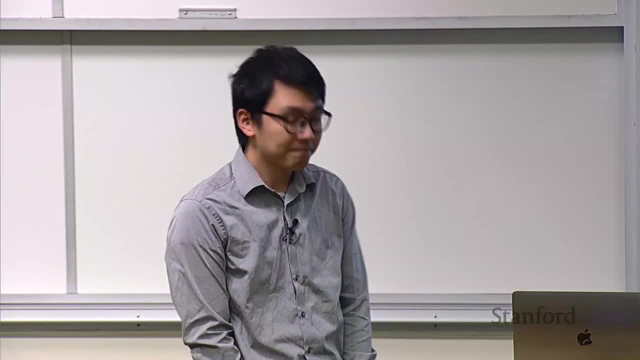 just in one step. So it all really depends, Yeah.